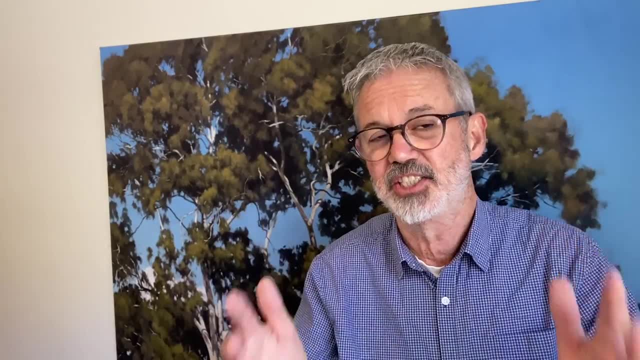 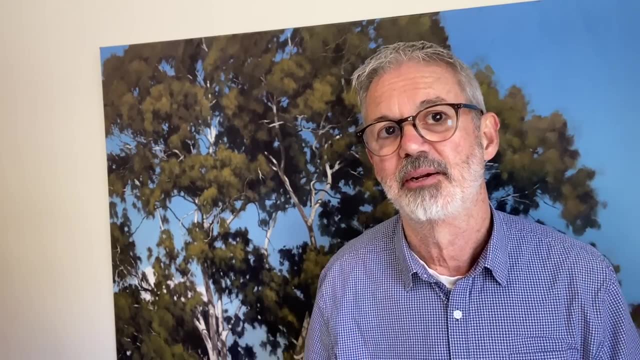 I really have to see what I'm looking at and just draw it accurately. I don't really need to understand anything of a theoretical framework and if I draw accurately it will look right. But in my experience, if I understand what I'm meant to be seen, it's easier to see what's. 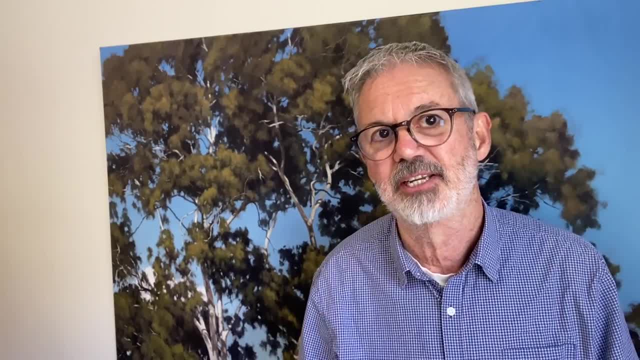 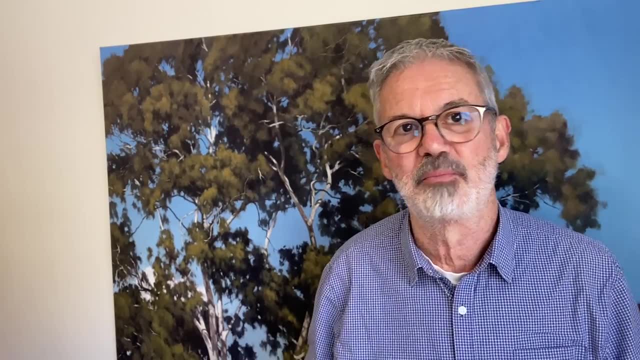 really there and therefore easier to draw it more accurately. And, of course, if I'm creating a scene for myself, I think it'll be easier to see the scene, And so the more I work on this, seen from my imagination- even a three-dimensional landscape, say, for a game, where the viewpoint 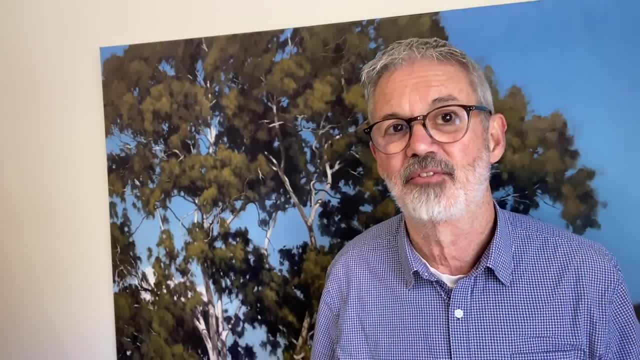 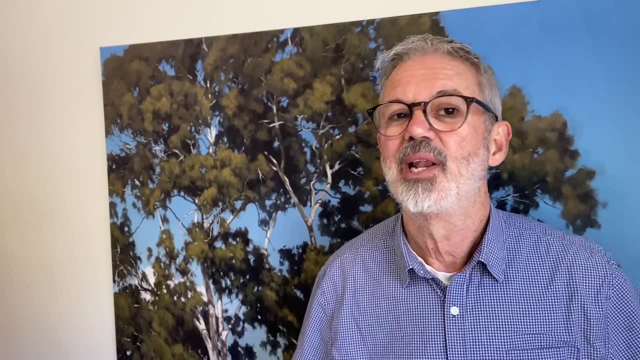 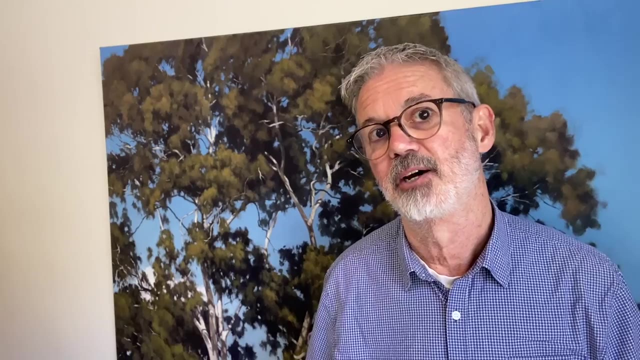 changes continuously, then I actually have nothing to copy from. And it's even more important to understand how these perspective principles work. My aim is that this video will help equip you to understand the situations where one, two or three-point perspective apply. 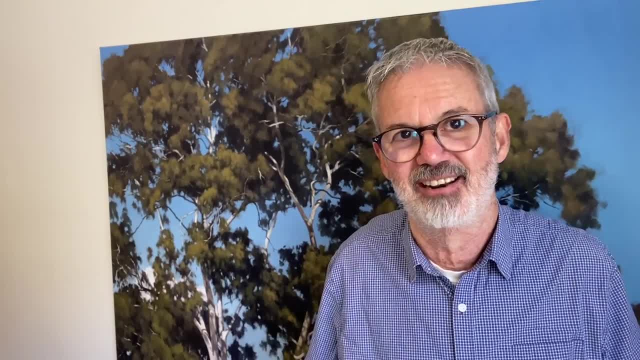 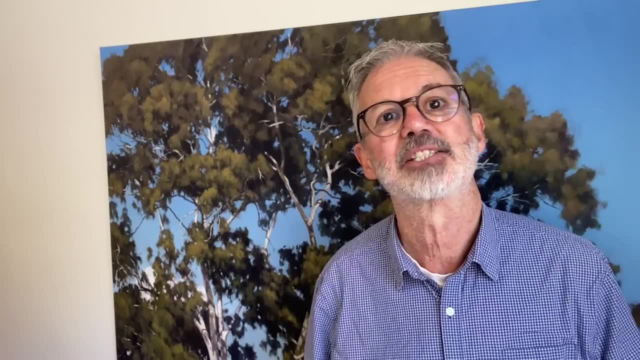 G'day. I'm Stephen Travers. If you've subscribed to my channel, thanks. If you haven't, and you've watched some of them and you think they're helpful, then please subscribe, please hit notifications, please comment, please do all the things that you know help grow a channel. 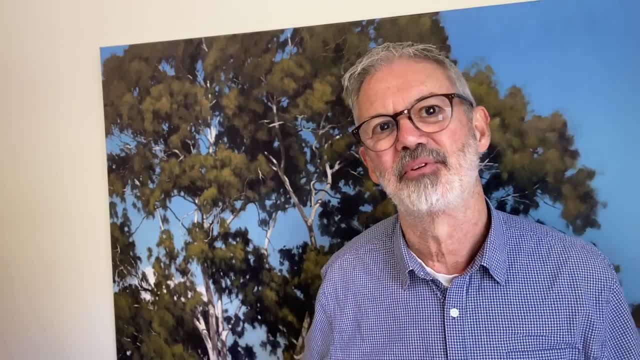 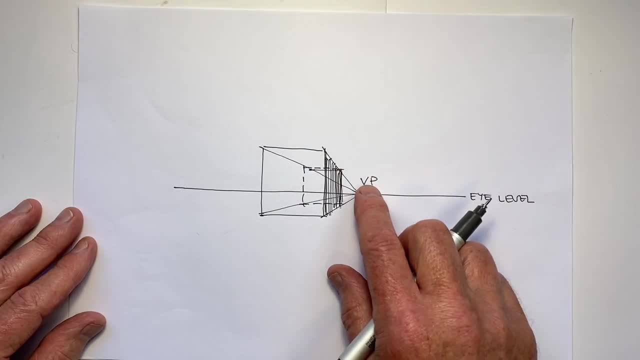 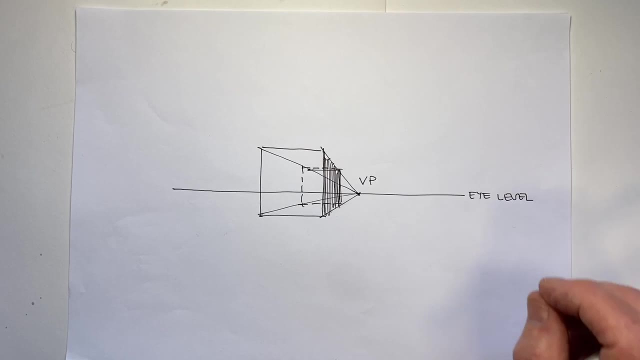 I'd really appreciate that. So we'll start with one-point perspective. When we talk about one-point, two-point, three-point perspective, the point refers to the vanishing point, the number of vanishing points that a certain view of a certain object will create. Therefore, in one-point, 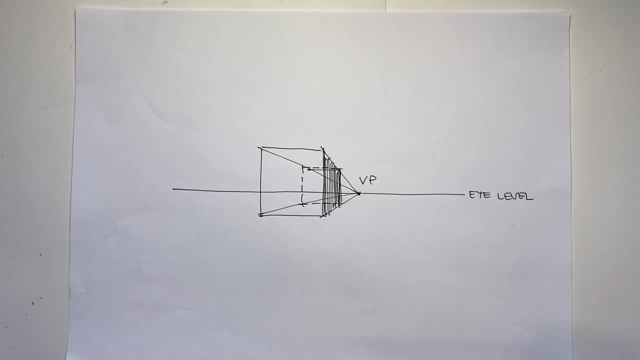 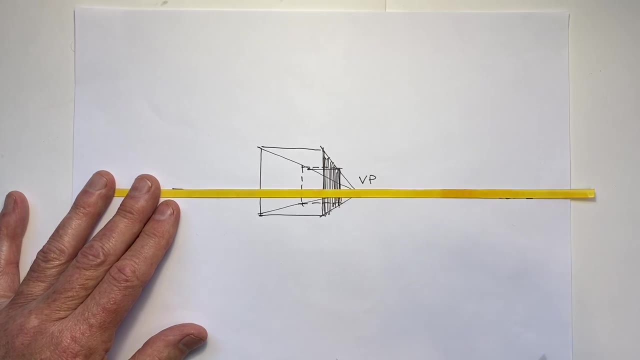 perspective, there is one vanishing point. The other thing we need to understand is that there is one vanishing point that sits on the eye level, and the eye level is the level of our eyes as we're viewing the object, or the level of the camera. So in this case, this is the point where 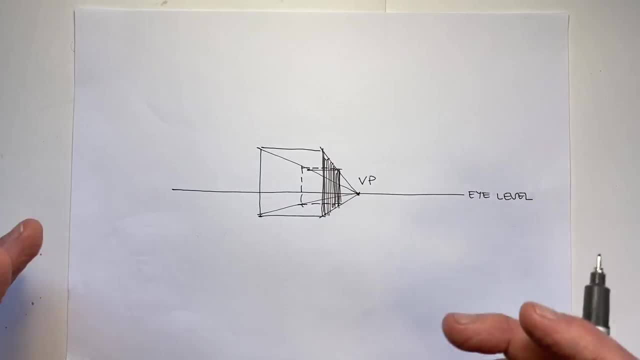 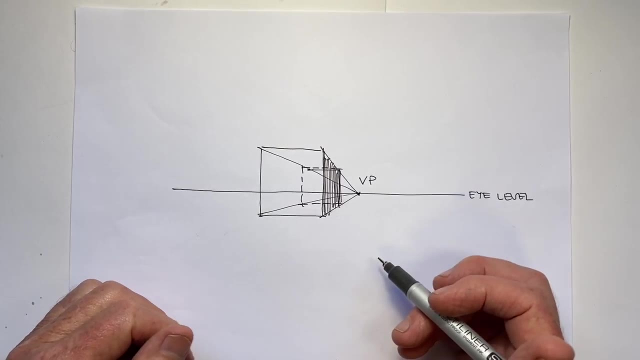 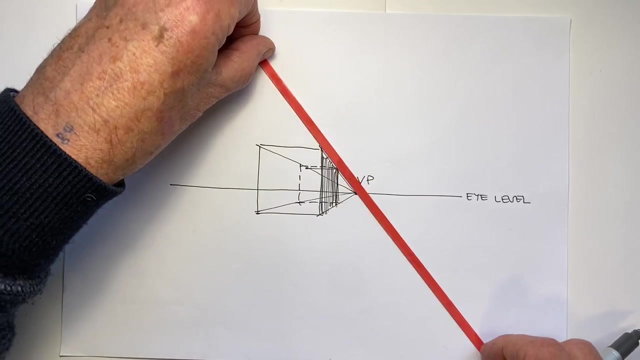 the camera was being held. And the reason why it is one-point perspective is because when we stand front onto an object, or almost front onto an object, then we pretty much see the front face and the angles of the lines at right angles all meet at a certain point on eye level. 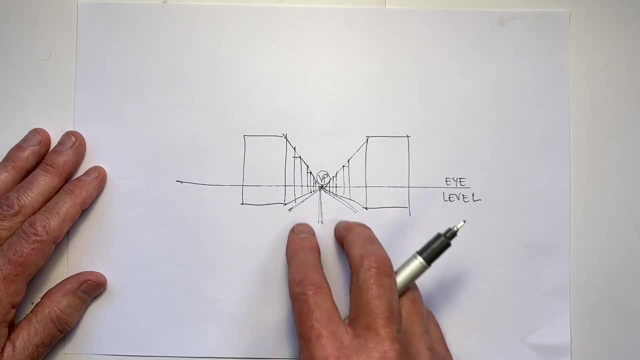 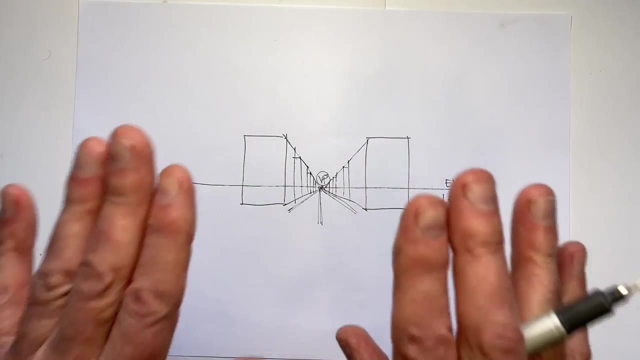 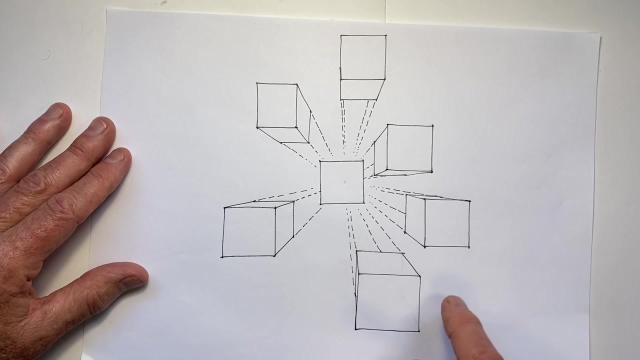 This is also one-point perspective, where it's this roadway which is the object we're directly in front of, but we're in effect the fronts of these objects. we're still looking at front on without any distortion. All of these objects are in one-point perspective, even though, for one of 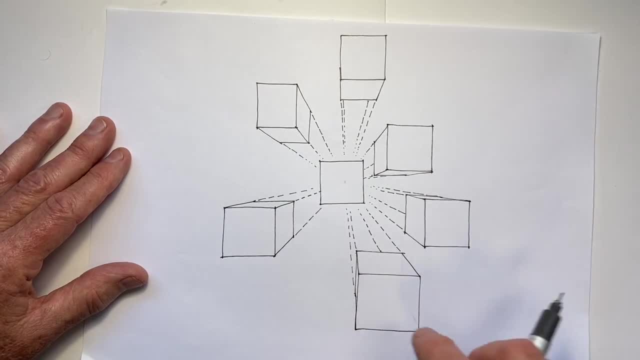 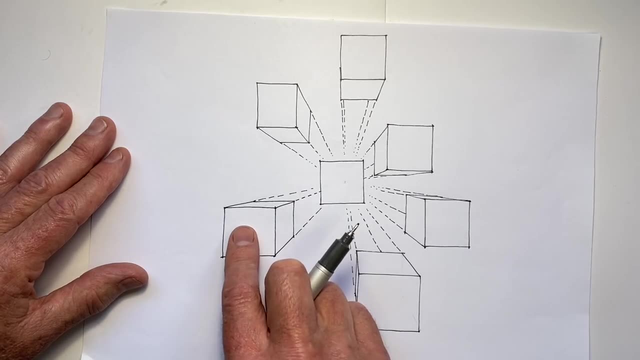 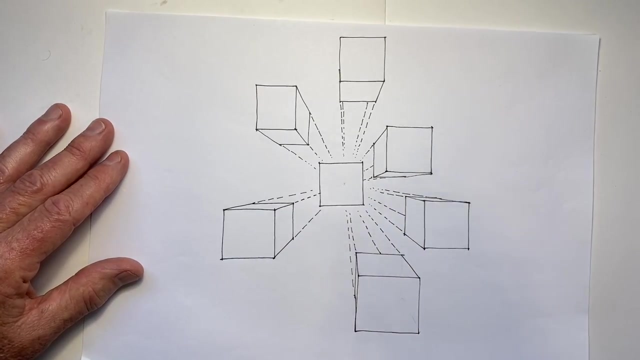 them, we're looking directly, square onto it. For others, we're looking square onto it. For others, we're looking square on, but down. others square on and up, others square on, but from the right, or others square on and up and from the left. Because, from this viewing point of these objects, 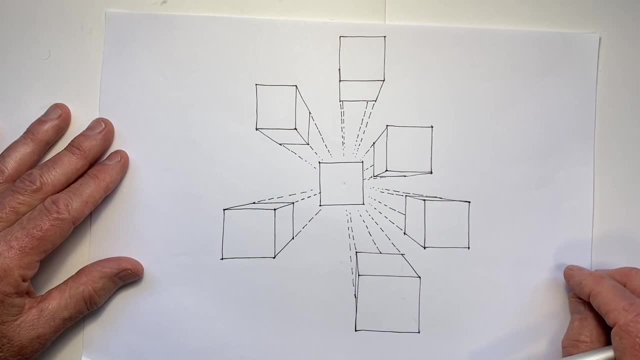 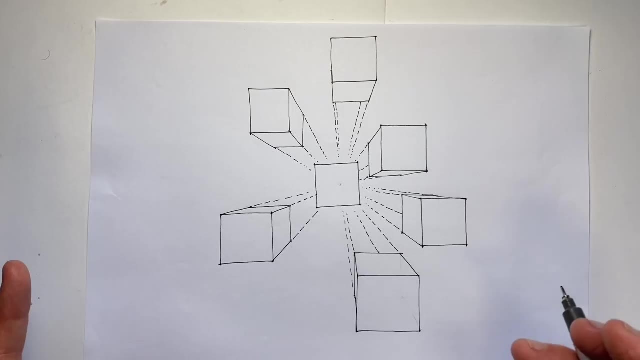 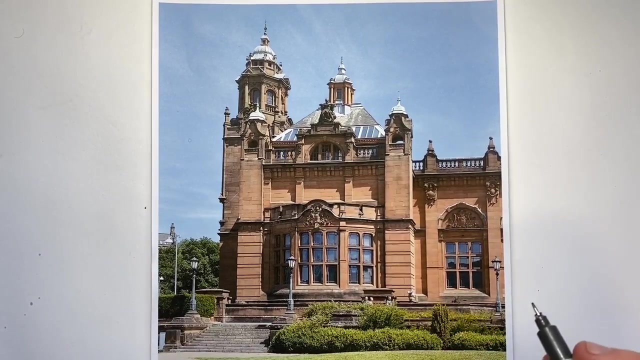 there is only one point that all of these lines go back to- one vanishing point. So we need to look out for one-point perspective when we're looking straight on at an object. Here's part of the Kelvin Grove Museum and Gallery in Glasgow. This perspective reflects this. 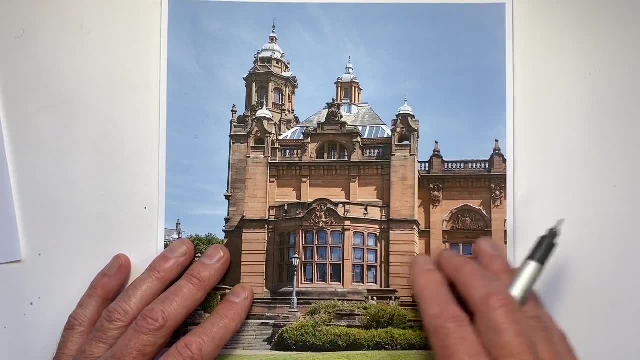 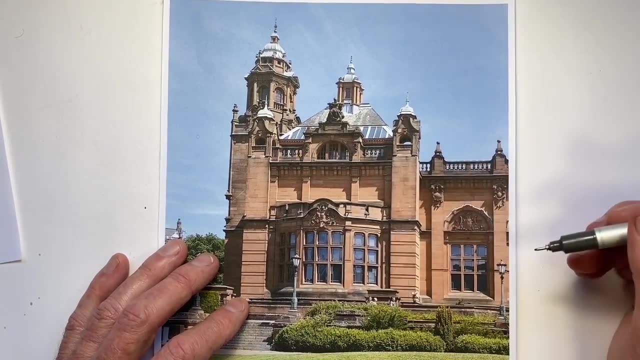 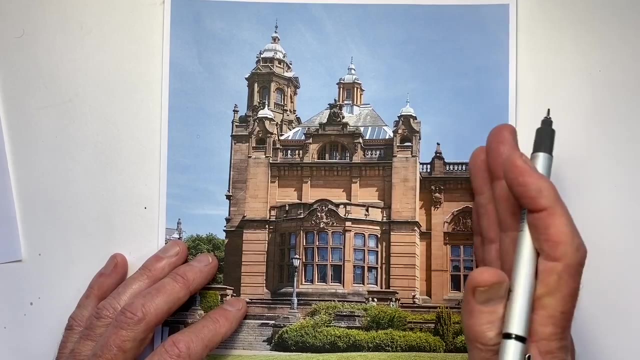 in that we're not exactly in front of it. we're slightly to the side and we can see there is a very slight perspective view of the side. If we were to stand back a bit and see more of the building, then at some point we would see none of this, and then if we kept moving to the right, 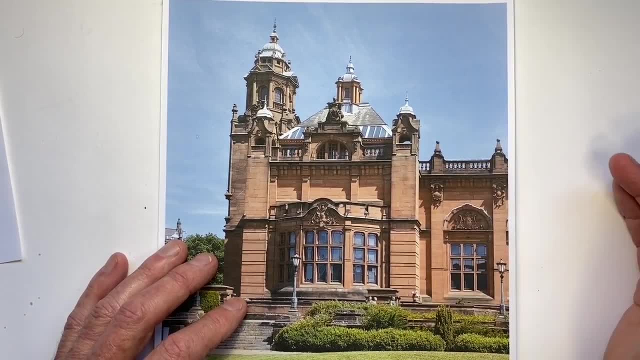 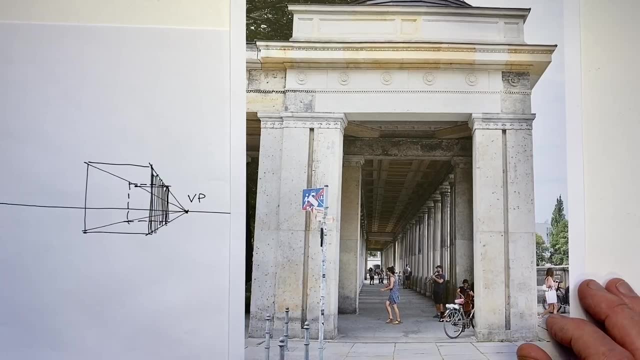 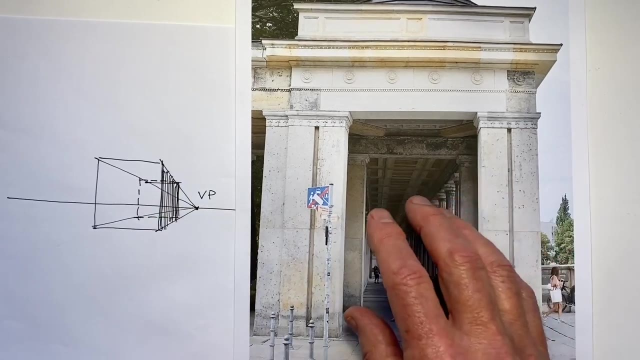 we would start to see something similar to this, but on the left-hand side of the front facing wall. Here we have the sort of example which relates back to this perspective model, except often with a building, this face is a wall and we can't see inside of it. In this case, because this is an open 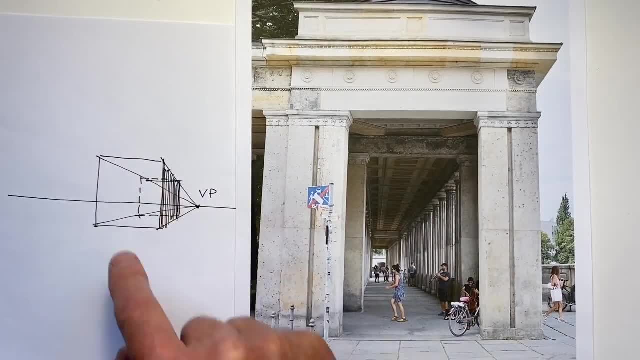 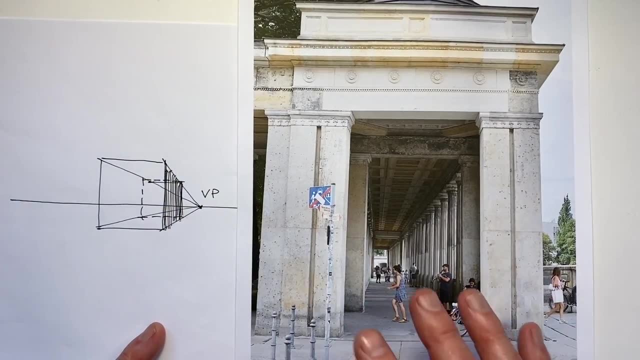 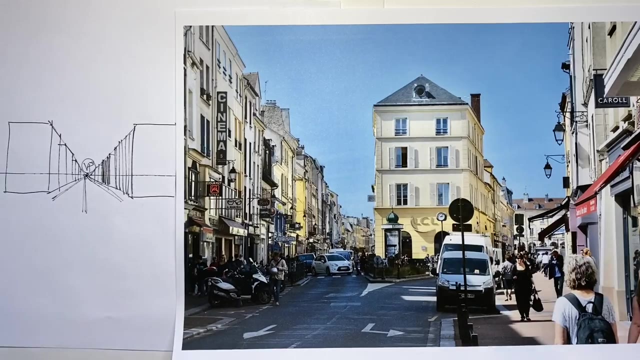 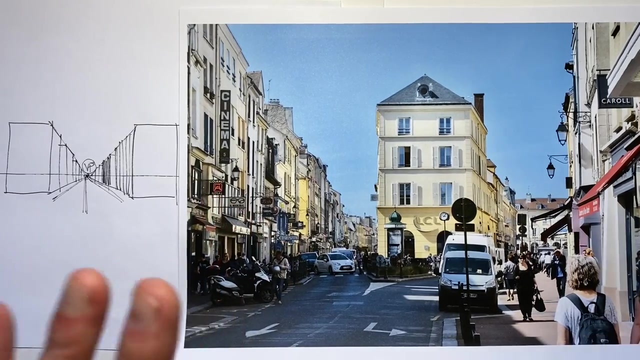 arcade. we can in fact see these lines as our theory tells us they're going to be there. So this model is also applicable if we're in an interior space against one wall parallel to the opposite wall. Our third example is a good example of how simple theory diagrams actually don't always apply in real life. Basically, this: 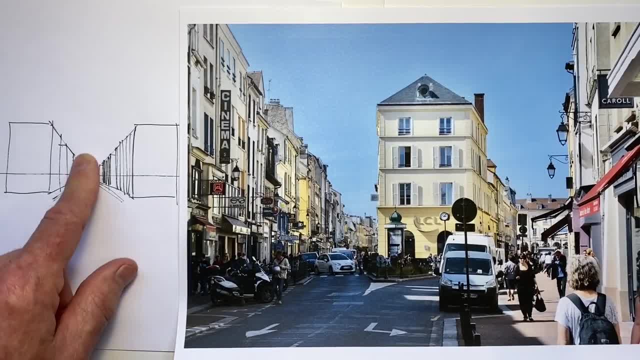 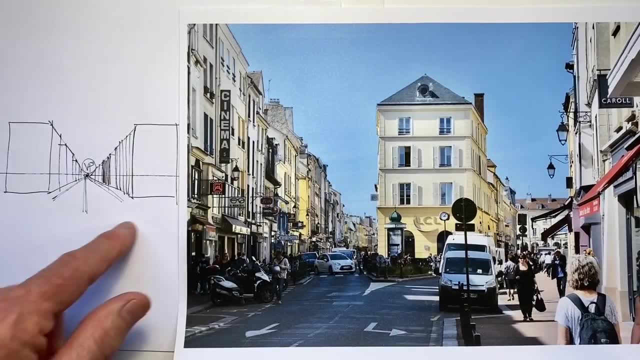 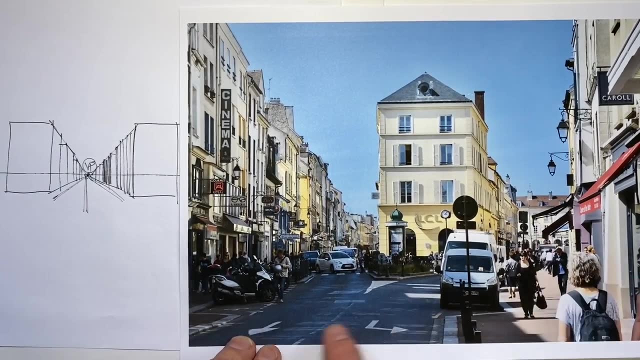 is a one-point perspective view. We're in the centre looking up a street and we have buildings on both sides who have perspective lines coming down. But this sort of perspective diagram always assumes that the ground is flat, and in this scene we can see that the ground does slope up. 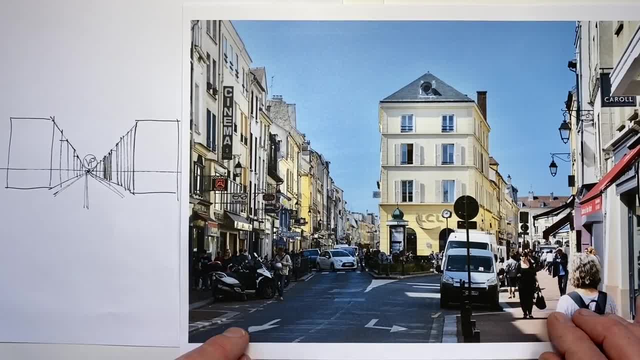 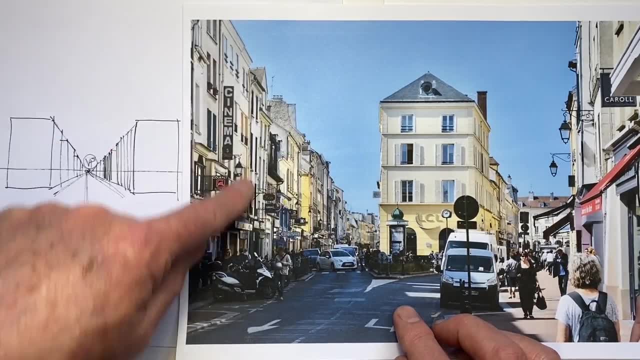 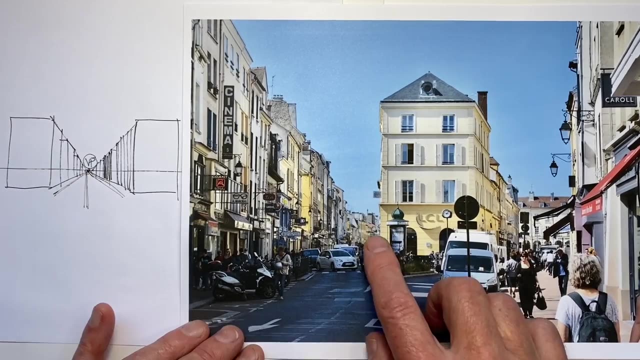 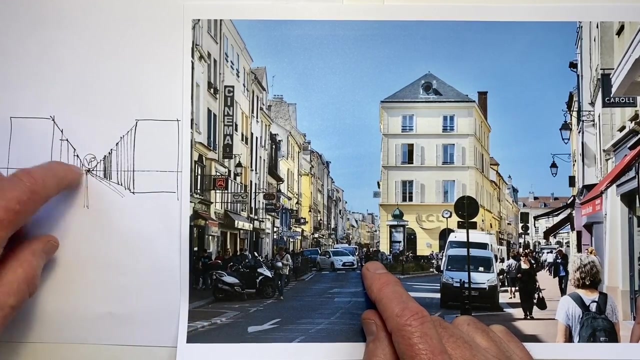 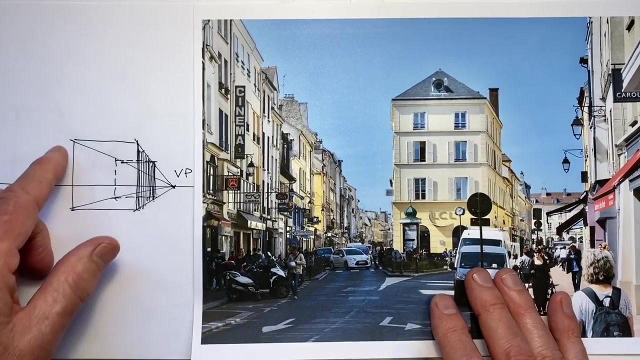 more so on the left side than the right side And both sides have perspective lines coming to the rift between all buildings but that tug of war. So we also see this is a one-point perspective as we look at the action and the pressure relief of that very small building. and then, because we're in the centre of this frame and the 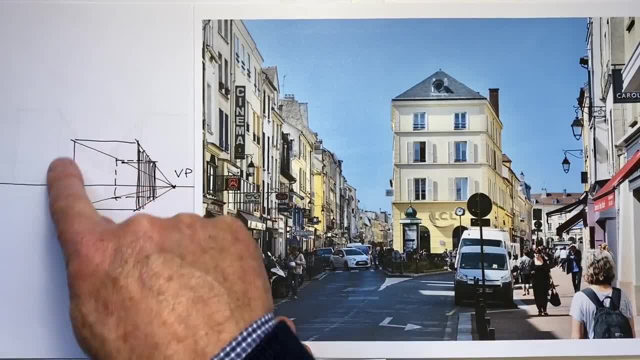 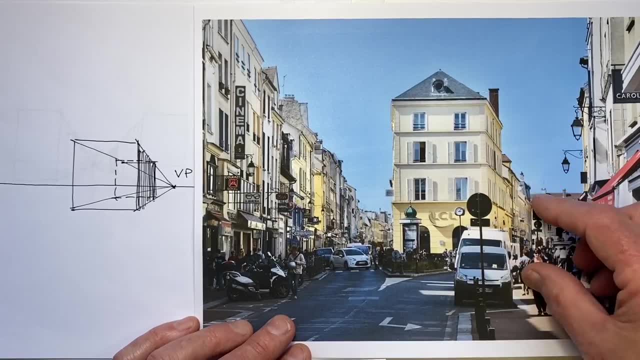 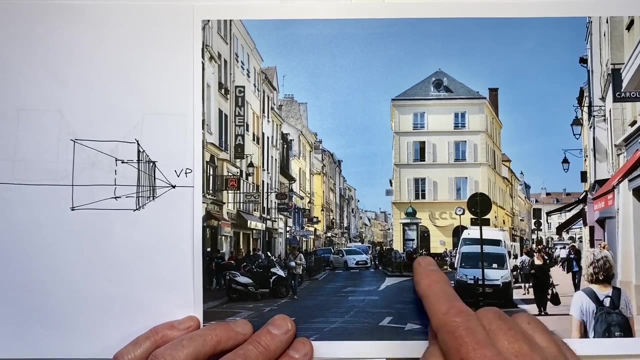 rise of the video front on face, which has minimal distortion, and we see something of the perspective of the side, and that same principle applies for the whole block on this side of the street. after this point the buildings veer around to the right to make room for this road here around the building and 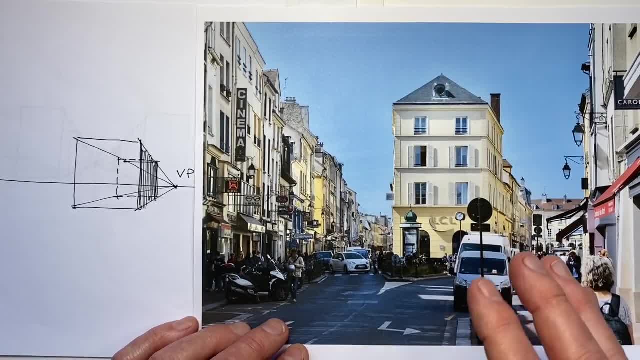 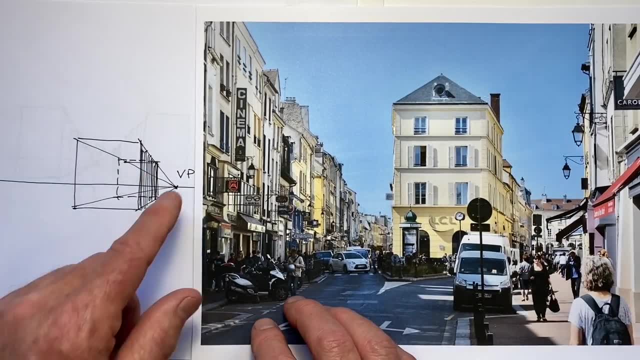 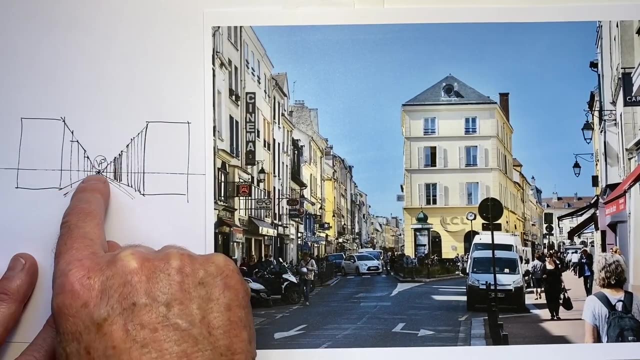 we don't see them anymore. so one really important thing to realize when we're trying to go from small theory diagrams to real life is that these are based on flat ground and that they're based on rows of buildings in a straight line where the road is the same width the whole way up and so 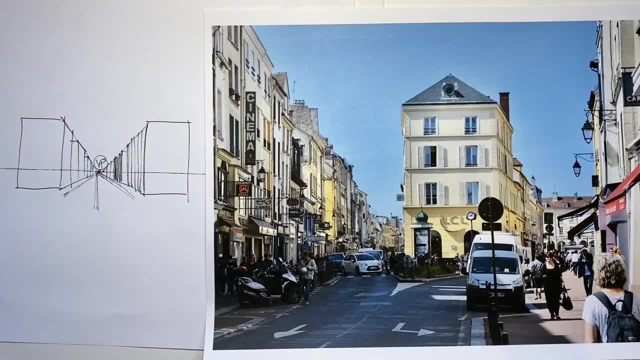 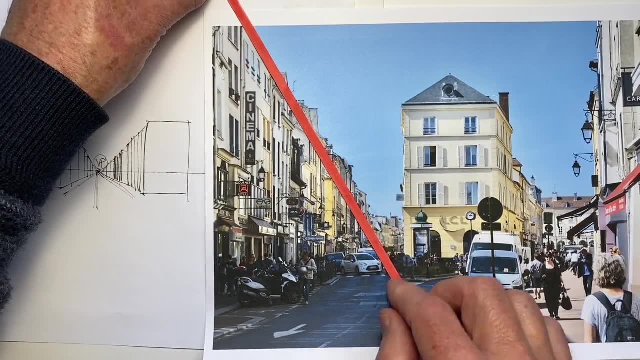 when roads widen or come in to turn a corner or a bend, that means that these perspective lines don't apply. this perspective line isn't applying to these buildings a bit further along, which isn't applying to these buildings a bit further along, which isn't applying to these buildings a bit. 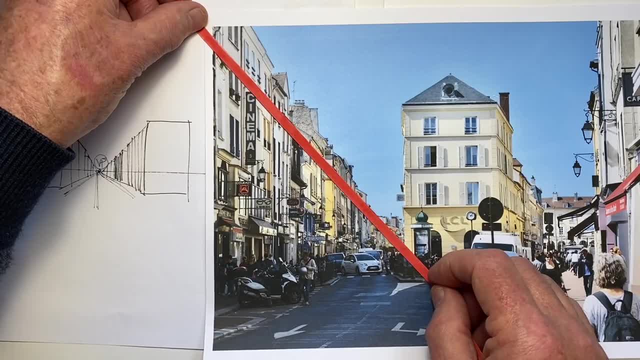 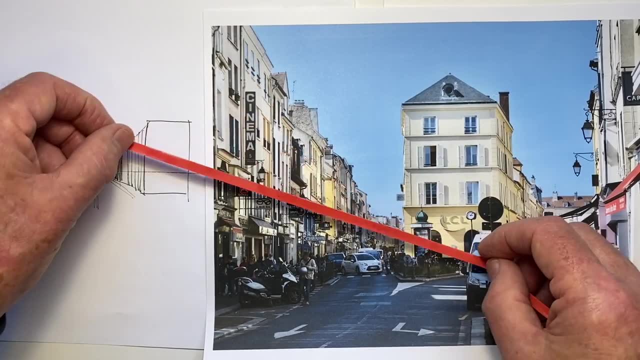 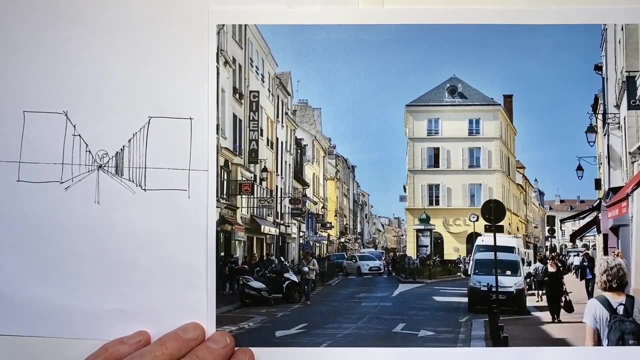 it is not just one line that we can trace down through all the windows from here to here. it's not just that the windows are at different levels, but the angles actually change. so if i'm on location drawing this, i know that this sort of effect is happening, but because i can see, the ground is not. 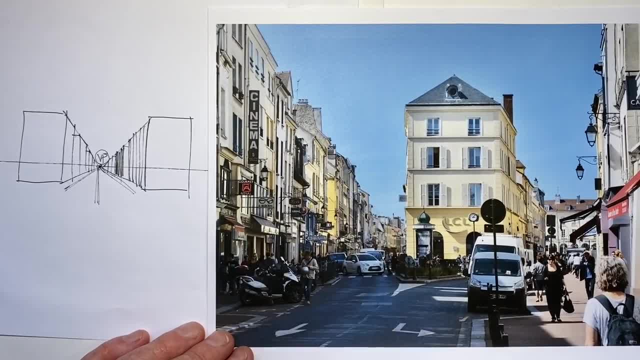 even, and this street frontage is not 180 degrees but weaves in and out. i know that it's not going to be as simple as this and i will need to observe these points carefully and if i try to draw this as if it were that i'll get into endless trouble, because i'll either have too much- 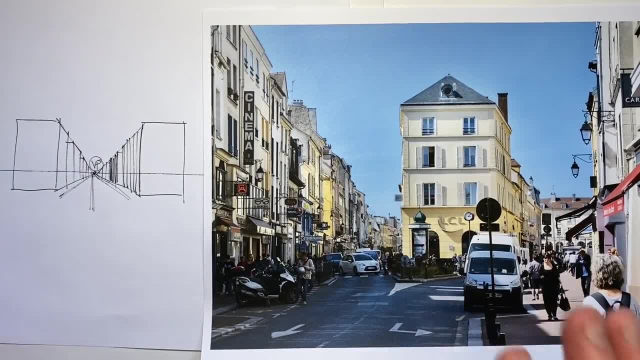 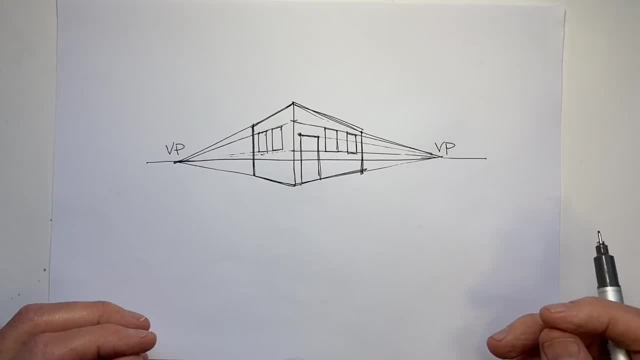 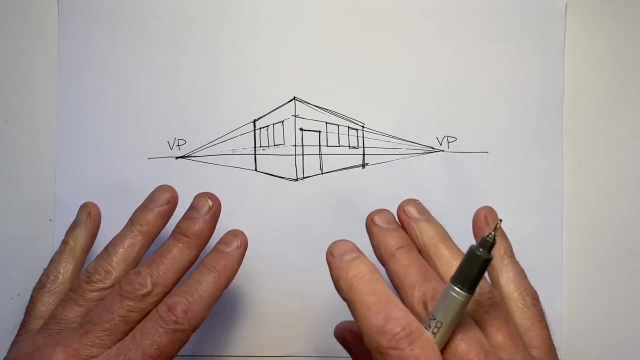 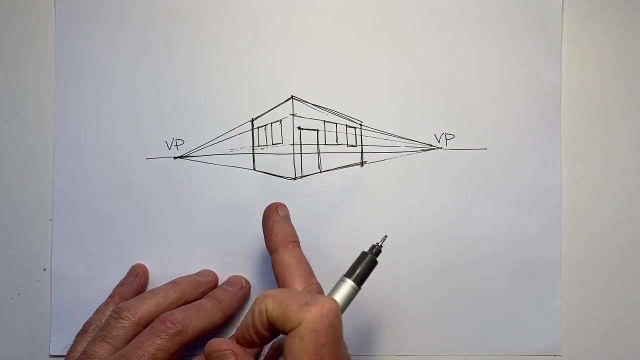 or not enough space to put the details into now. we'll look at two-point perspective. two-point perspective is probably the perspective most people are thinking of when they hear the phrase perspective. it's where we have two vanishing points on our eye level and we get two-point perspective when we're not standing front on looking at an object, but we're 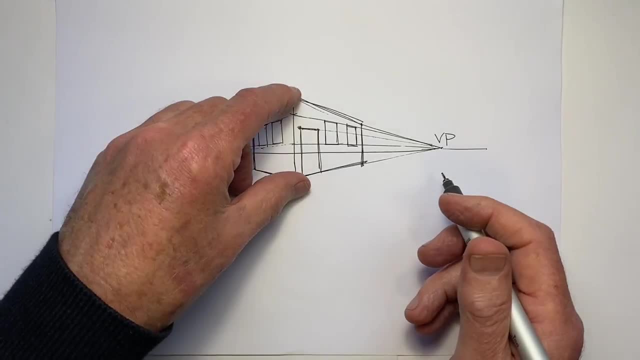 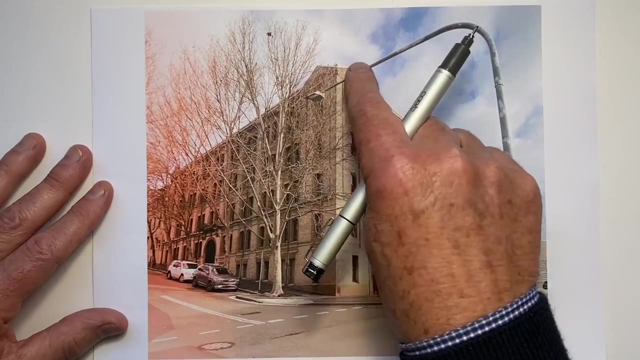 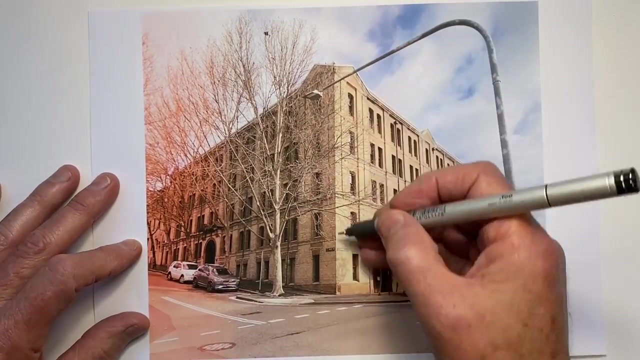 standing looking at it from an angle, and so each side has its own vanishing point. in its simplest form, it's a box. so here we have a building and we're looking at it at an angle and we're standing pretty much straight onto this side and, because this is a right angle street, hidden a little bit. 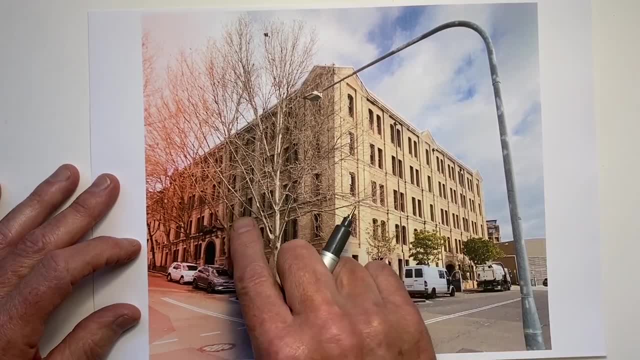 by the fact that it goes uphill on the left. here we're facing these side walls at pretty much the same angle and because of that, because of the side walls, it's going to sing out out of the right side: the side walls that are going to be the right side and the side walls that are going to be the 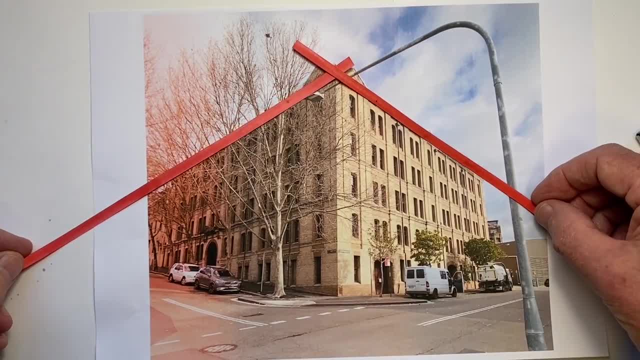 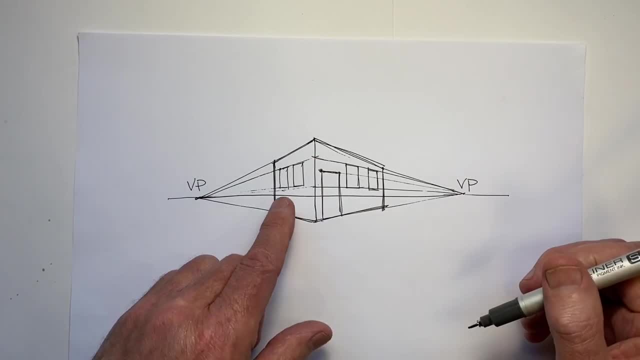 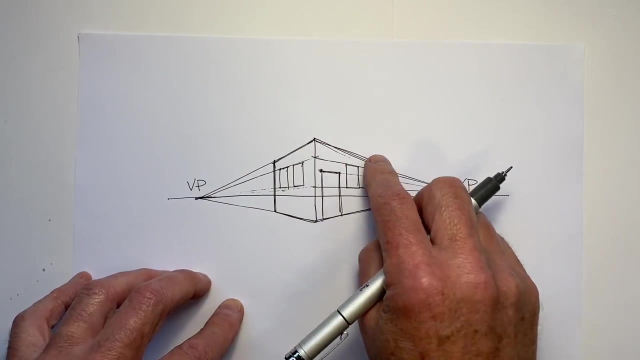 that The perspective angles are very similar. However, if my example is more like this diagram, where one wall is moving away from us more than the other, it will have a greater angle here and here than on the side where we're a little closer to being front on. So here's an example. 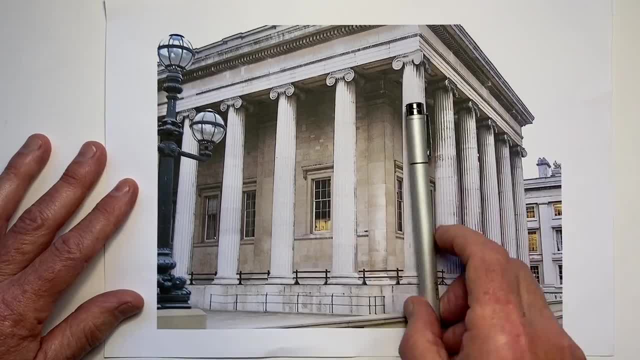 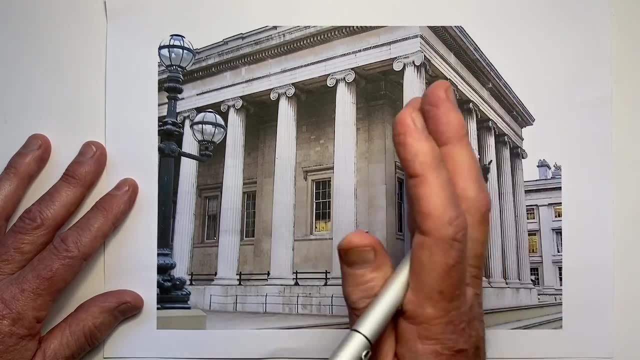 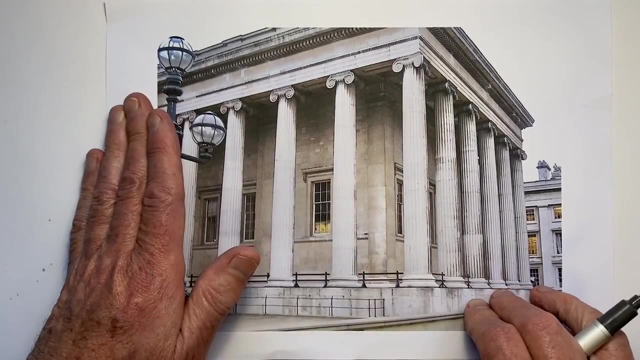 of that. Here we have the corner and we can see actually more easily here than in the diagram that this wall is moving away from us as we go along the wall at a much faster rate than this wall which, even though it does still move further away from us as you move along, it doesn't move as 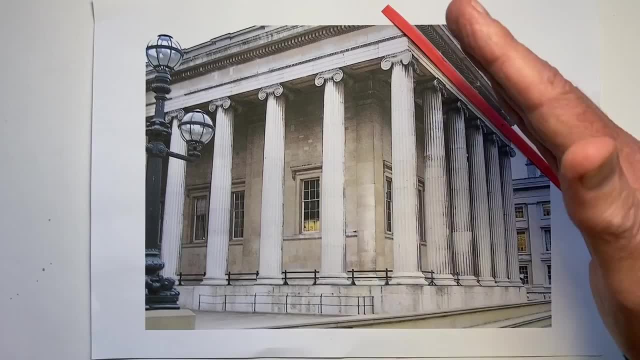 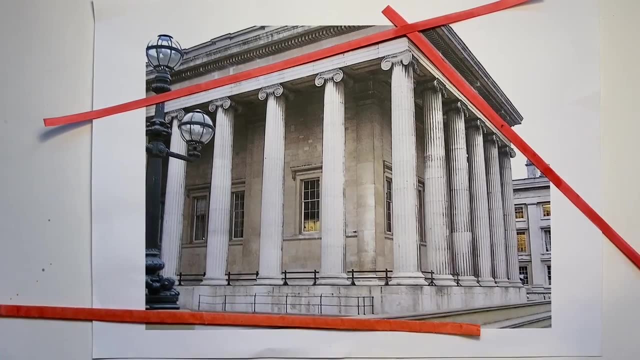 far, and therefore this angle is a steeper angle than that one, And the same applies at the lower end: This angle is not as steep as this one, and this is a really important conversation. So we need to think about this concept again, because if, when we're drawing, we make this angle, 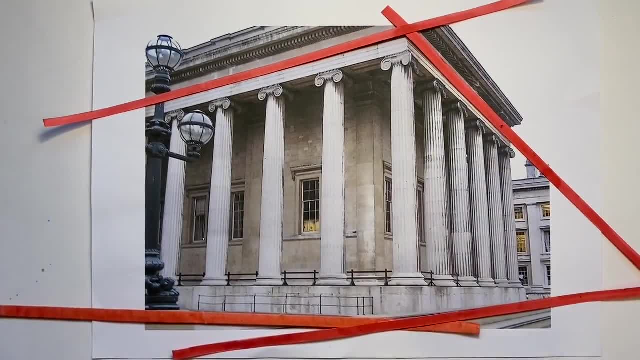 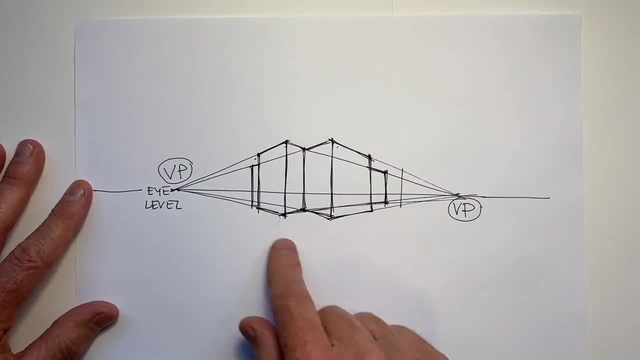 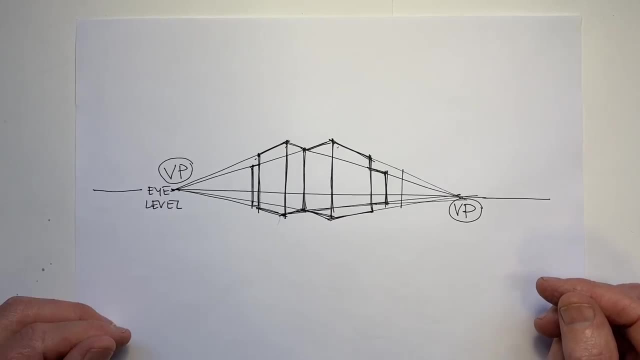 or this angle too steep. in effect, we push the building further away from us more quickly than is in real life. Of course, buildings don't have to be a box. Many buildings are, in effect, a series of boxes attached to each other in various ways, But we still have our principle that all the 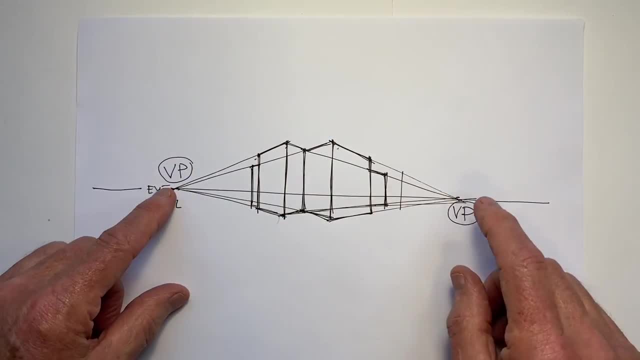 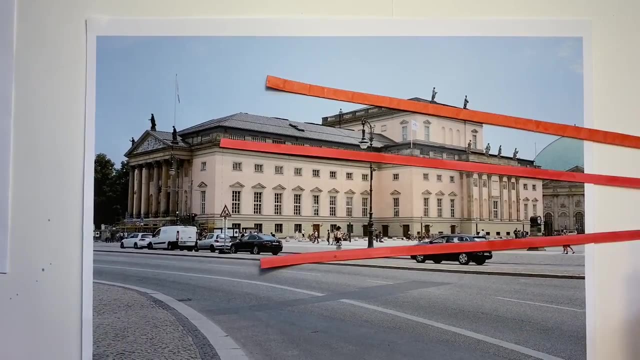 vertical lines at their corners go back to one of two vanishing points. So if we're drawing a building, we're going to have two vanishing points on eye level. This building is a good example of that. Off to the right the angles of perspective are quite shallow because we're more front on to 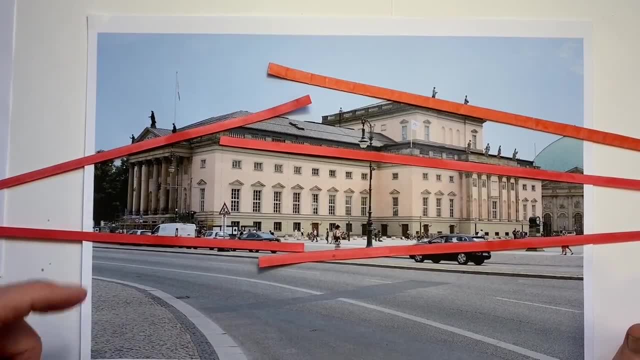 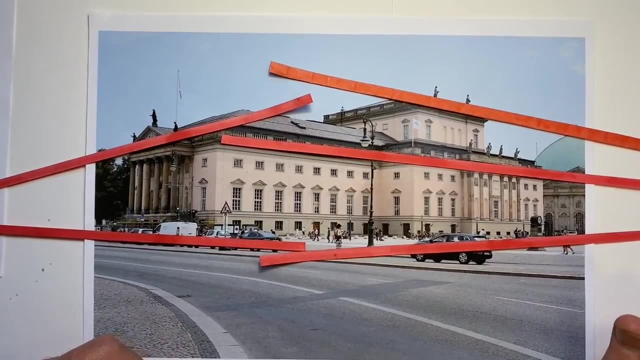 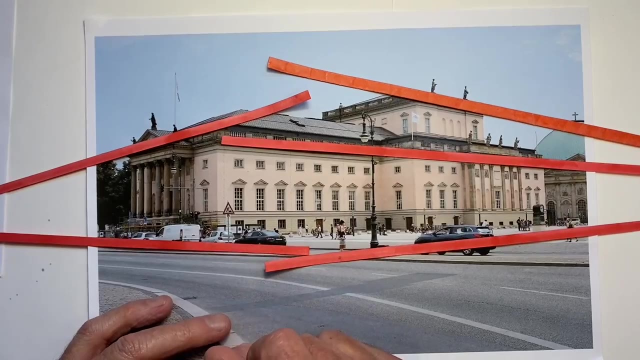 this long side Off to the left, the angles are steeper because this side of the building is sloping away at a steeper angle than this side And, of course, this wall and this wall and this wall all line up with the vanishing point for this wall. One important point to note is that the 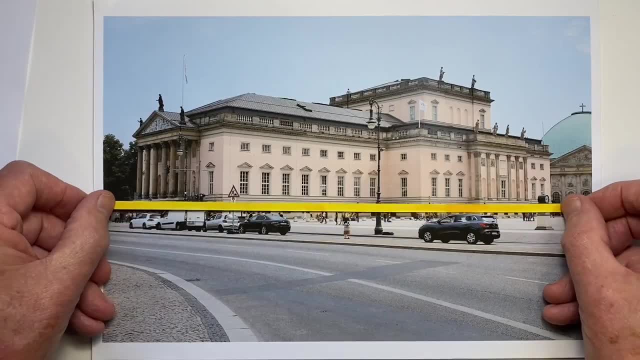 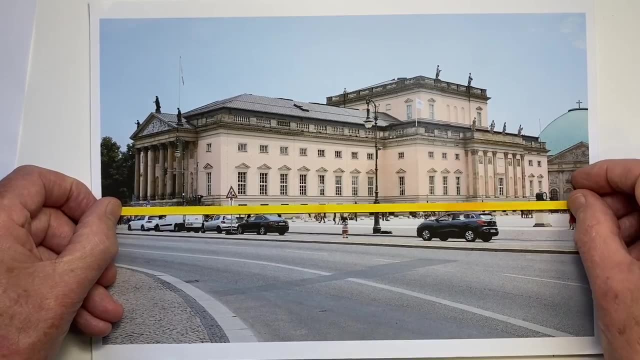 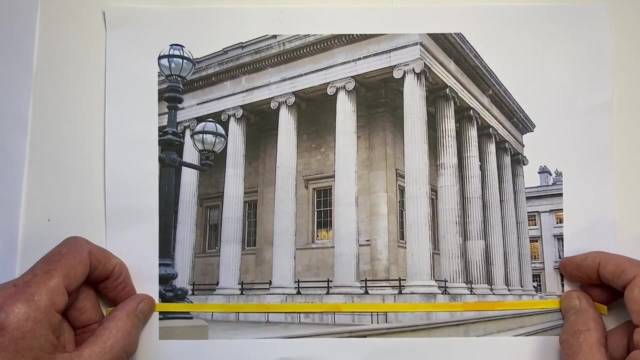 in these three examples. eye level is quite low Here because this ground is flat. eye level is actually the eye level of the people, So eye level is relatively very close to the bottom of the building. Eye level is here in this example That may look too low for the building, but what that? 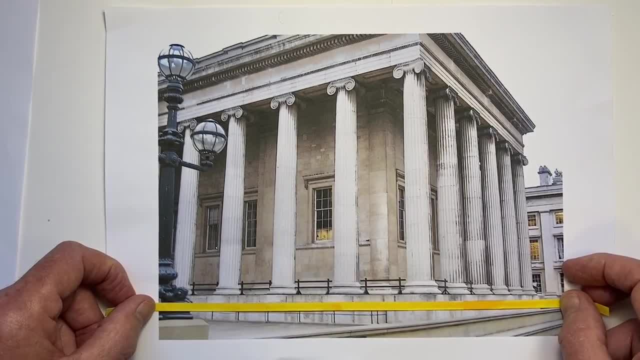 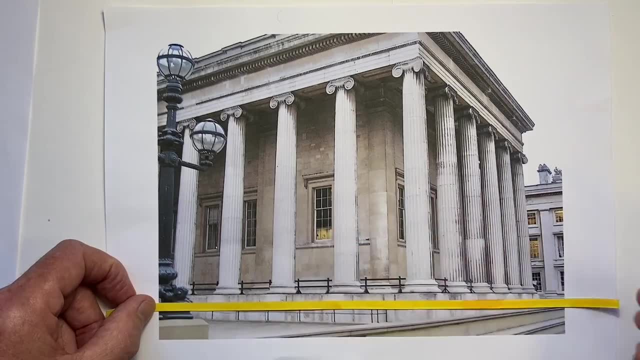 means is that I was standing on a lower level than the base of this building. Eye level is where horizontal lines appear straight, regardless of where I'm standing. So if I'm standing on a lower level than the base of this building, I'm not going to be able to see which side or part of a building 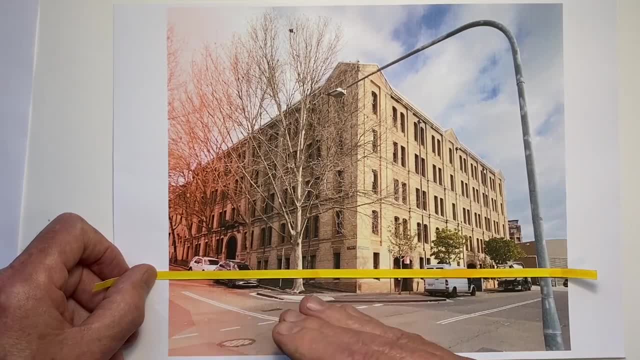 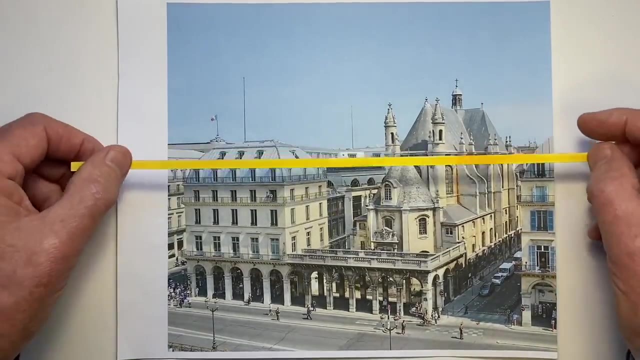 they're on. Eye level is low down. It is disguised a bit side by the fact that this is a sloping street. But I have a video that's particularly to do with perspective on uphill sloping streets. So we'll finish two point perspective by looking at this example, where eye level is very high in. 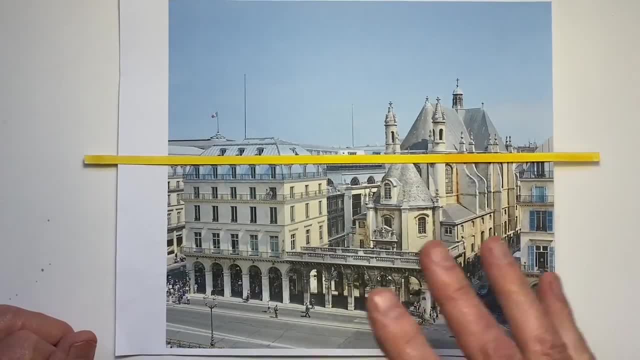 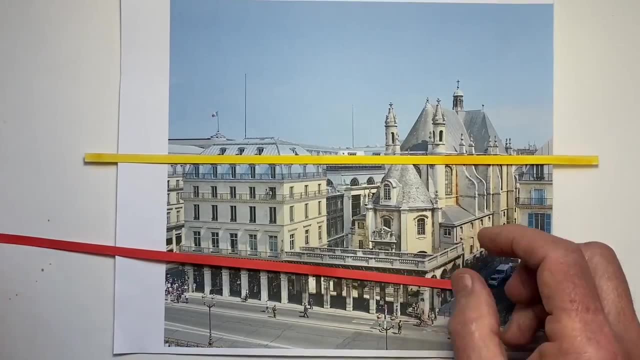 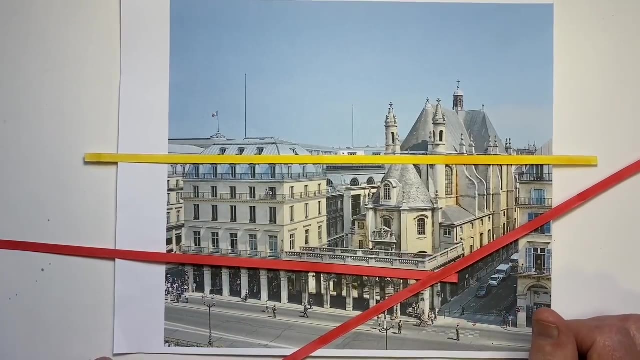 the building. In fact, eye level is about here and it can be this high because I was in an upper floor taking this photo through a window. And this is also a good example of how, if we're more front on in two point perspective, the angle. 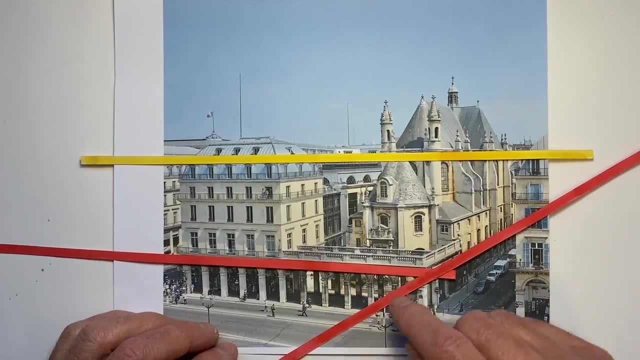 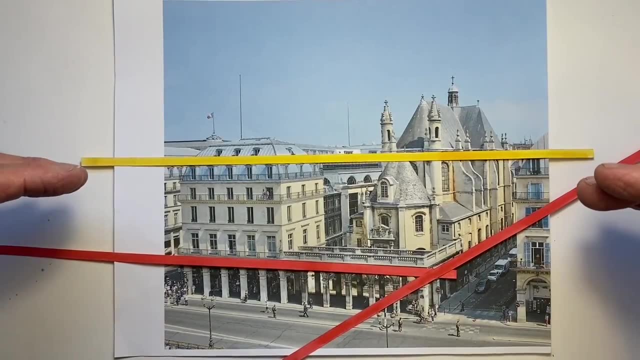 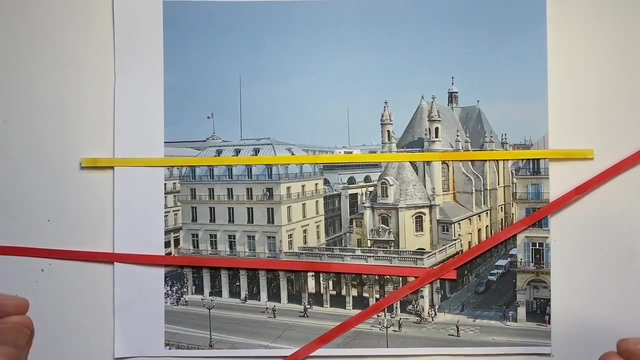 is shallow. If a side of a building slopes away from us more steeply, then the perspective angles will be greater. In this case, almost all the perspective angles are under eye level, but the rules still apply. Again, with two point perspective, it's based on the assumption. 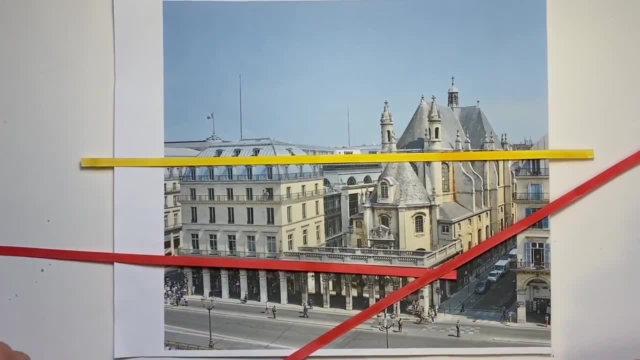 that the perspective angles are lower than the eye level, So if I'm standing on a lower level, that the streets are straight, that the buildings all line up on the same level and that the ground is consistently flat. Finally, we'll look at possibly the trickiest of all, and that's three. 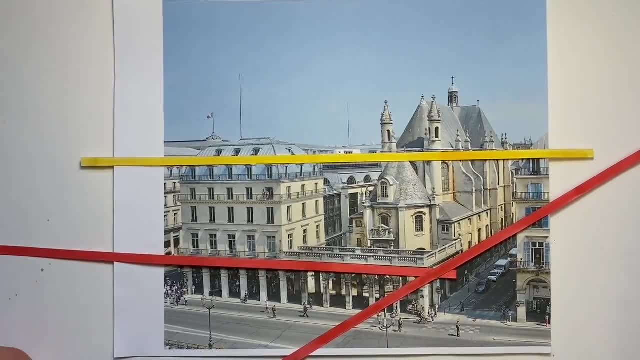 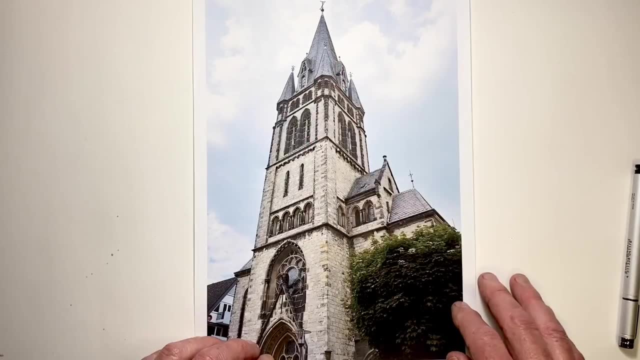 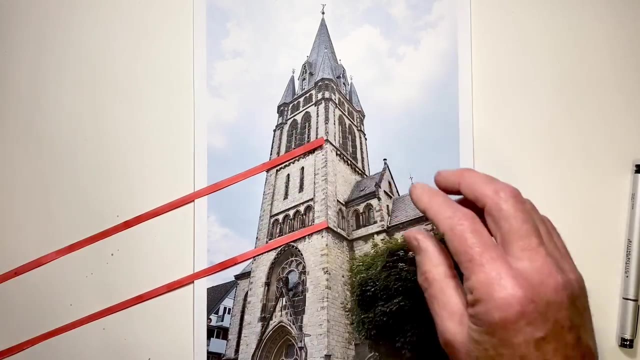 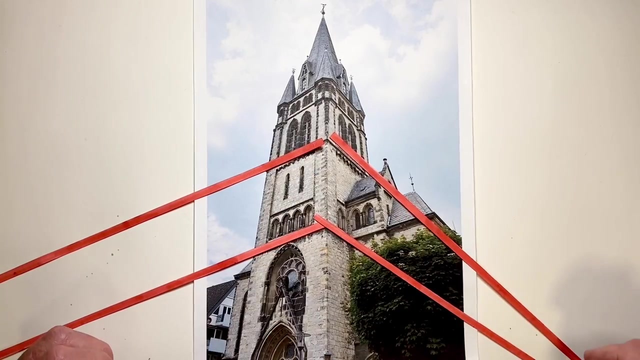 point perspective And there's a few things to consider with that. This is probably the most typical three point perspective image that we see. Here we have a spire of a church In three point perspective. we have our normal two point perspective. We have one vanishing point off to the left, one vanishing point off to the right, But we can see. 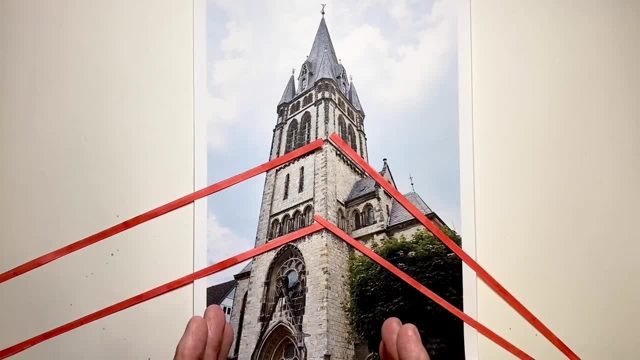 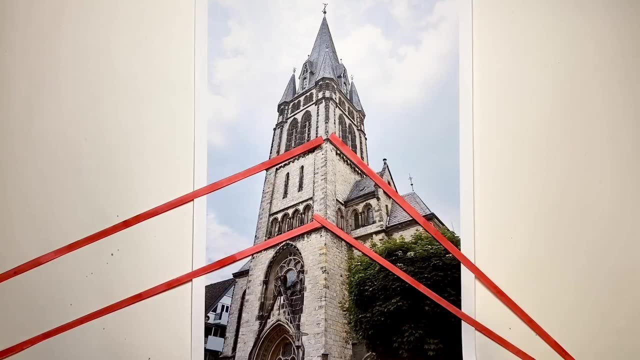 from the shape of the spire, that there's another vanishing point above: Although the center line is straight, the side lines angle up and that if you were to continue them, they would meet at some point. And that's the third vanishing point. And while we have an eye level on the horizontal plane, 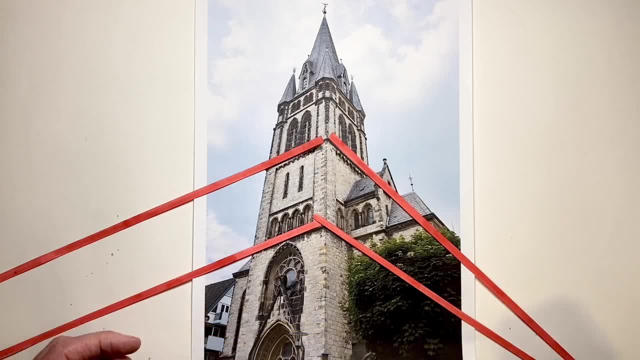 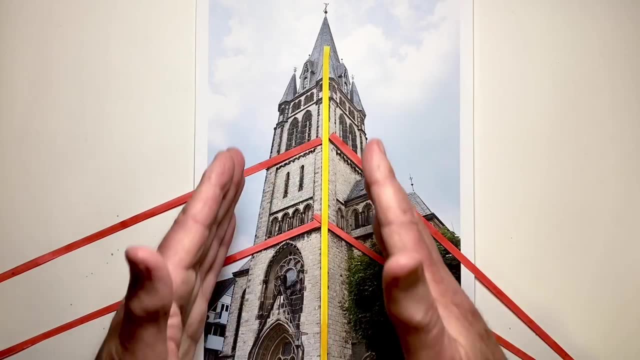 which is actually below the level of the spire. we have another vanishing point above, And that's this photo. We also have a vertical eye level And it's on this line that our vertical perspective lines will meet, Just as horizontal eye level is at the level of my eyes as I stand looking at. 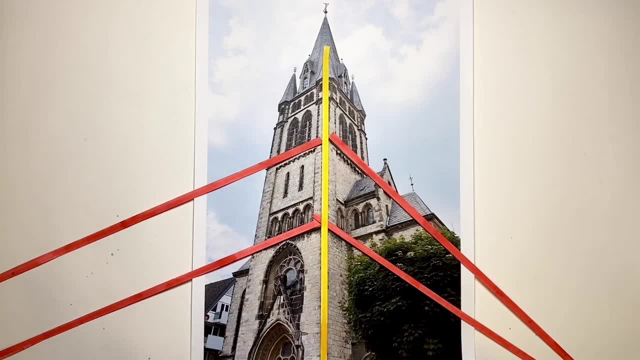 something vertical eye level is directly in front of my eyes. But we do need to be careful with photo references because if they've been cropped, then a part of a photo that possibly was on the left hand side of the picture is going to be cropped, And that's the third vanishing point. 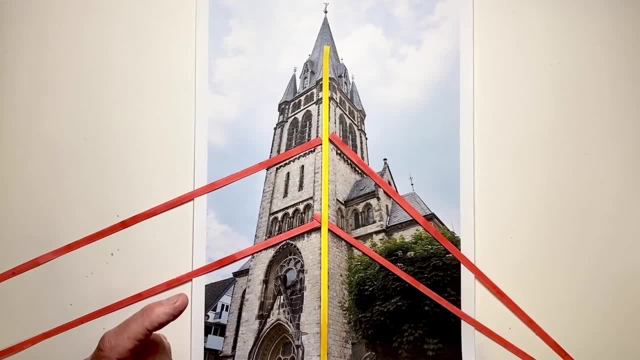 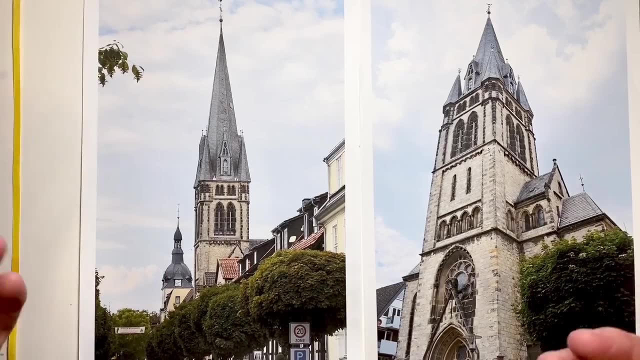 So now we can see that the vertical eye level on the right side may not have any true verticals in it, because the part of the scene that had the vertical has been cropped out Here is a view of the same tower, but from further back, And so the vertical perspective isn't really apparent. That's the 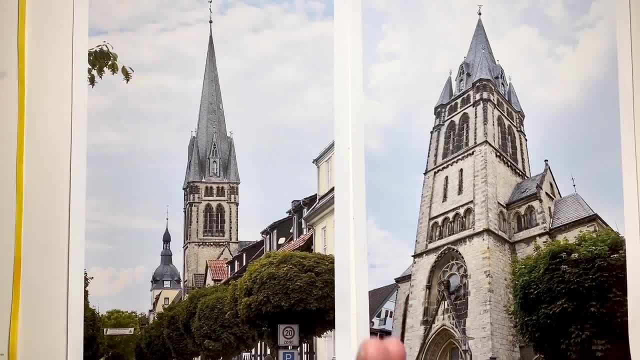 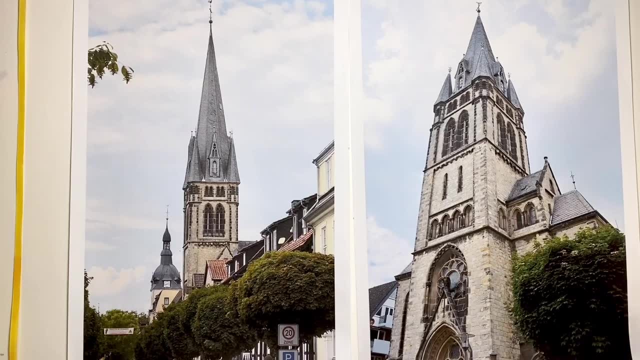 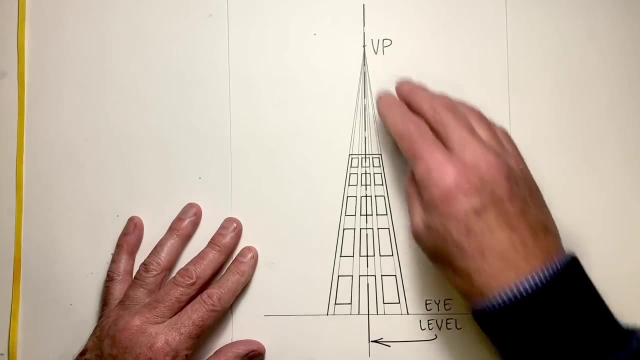 other point about vertical perspective. We get it with something very tall when we are very close to it, And so it has a sense of looking up or looking down. The taller it is, the further away we can be from the camera. But we need to have a sense of this angling to a point. Here's a simpler view. 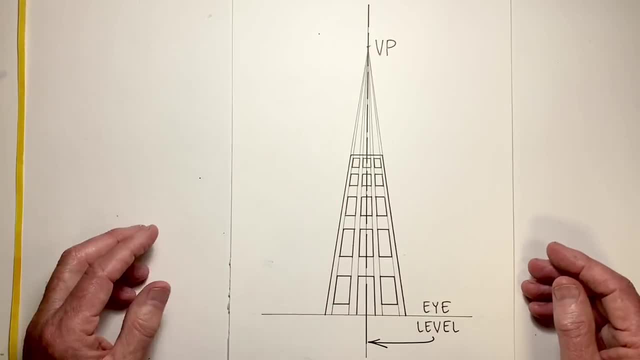 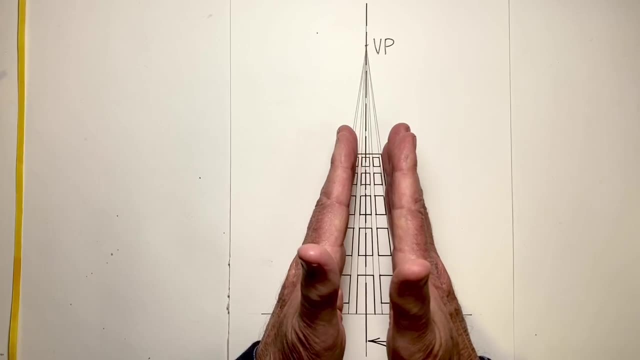 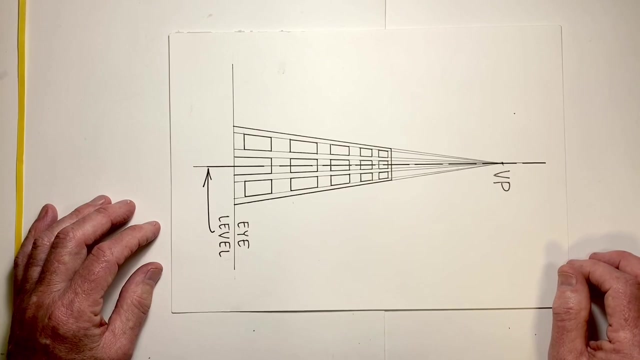 where we're looking straight onto the building, We're not looking at an angle as in our spire example. The vertical eye level is our one true vertical line and the perspective lines as they move away from it angle more and more in exactly the same way as they do in two-point perspective on one side. 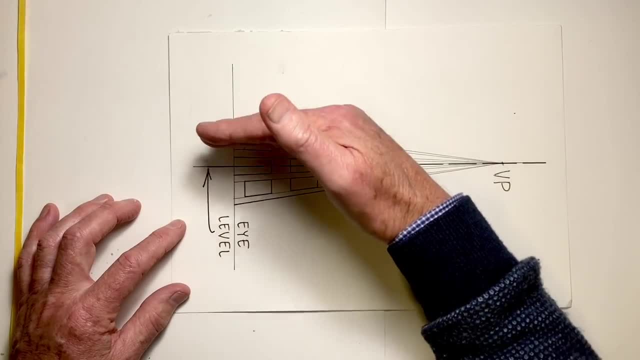 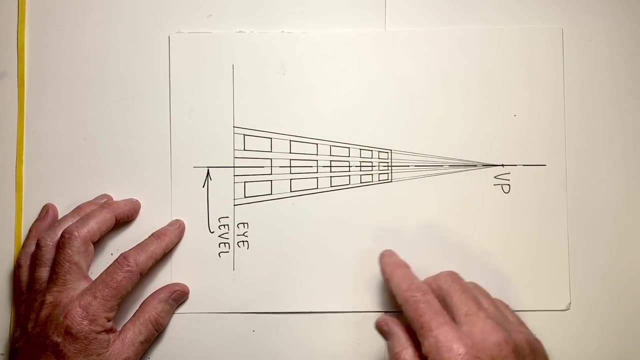 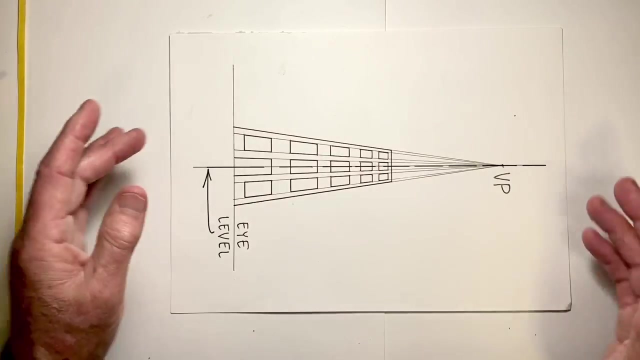 Where we have eye level, and as the vertical eye level changes, the angle is going to change as well. perspective lines move further away, above and below eye level, the angle increases. The other thing just to notice quickly is that just as we have foreshortening in perspective, which is the visual compression of what we're 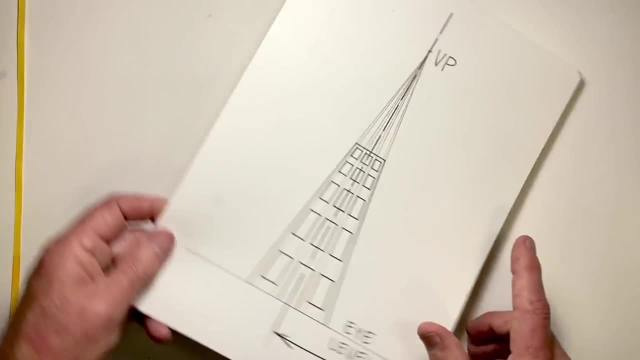 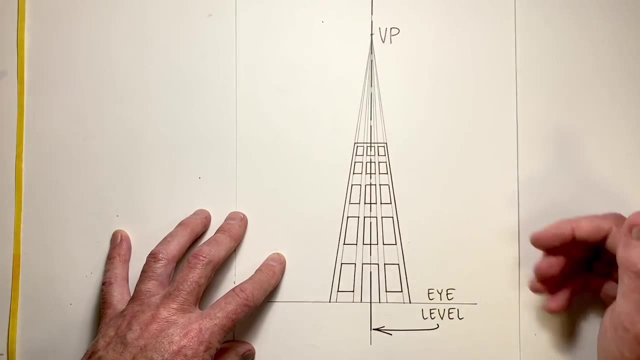 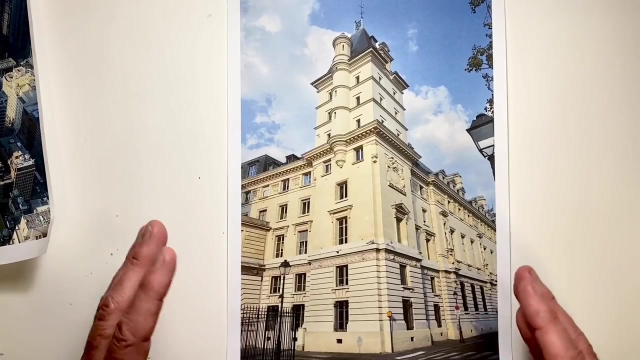 seeing as it moves further away from us. exactly the same thing happens on the vertical Vertical perspective. foreshortening means that as we look up a skyscraper, windows that are all the same size that appear compressed as they get further away. Vertical perspective happens on buildings as we look up, but 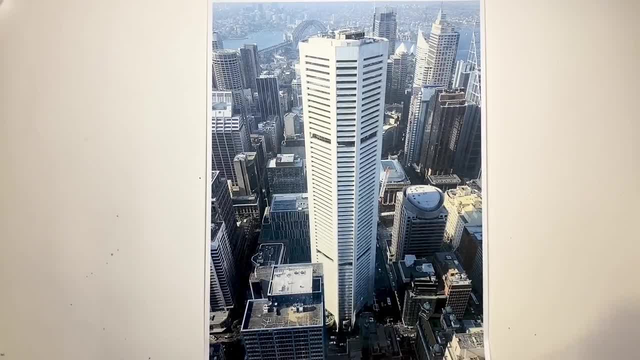 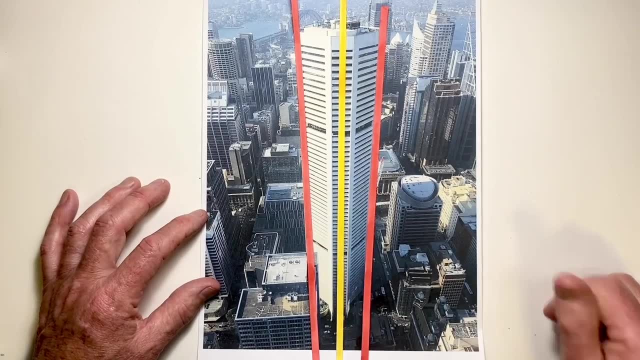 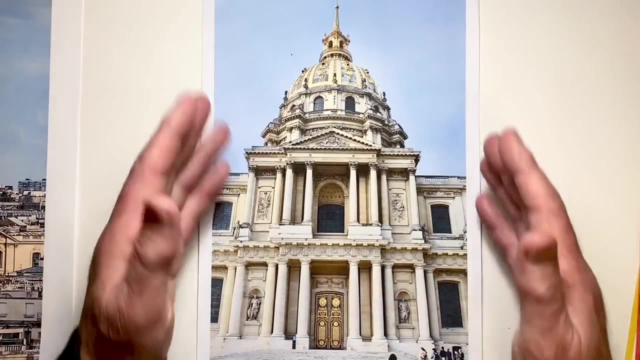 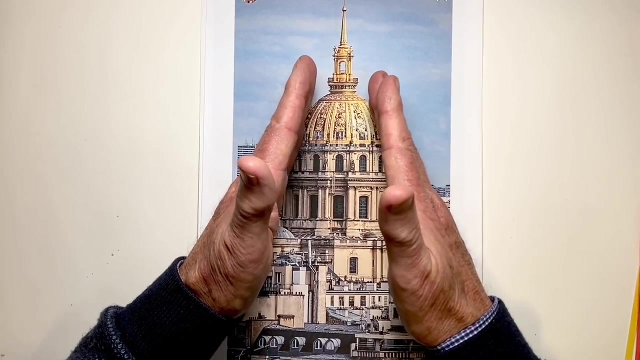 we also see it on buildings if we're up high looking down, as in the case in this Sydney skyscraper- and remember we see this effect when we're relatively close and low down to a tall structure. If we move higher up and further away and our perspective, vertical lines become. 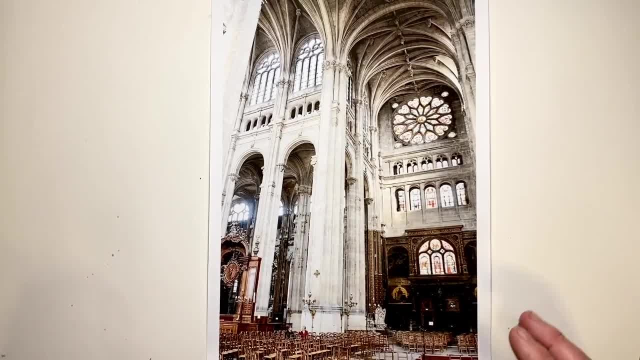 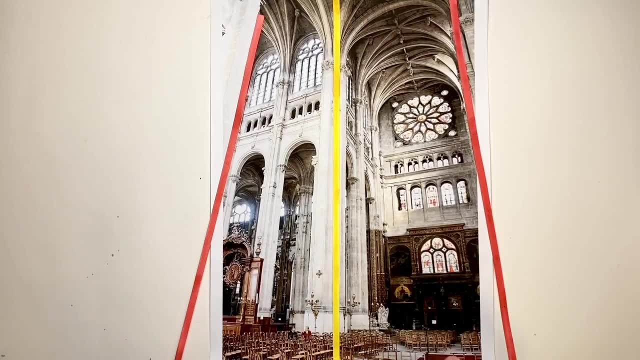 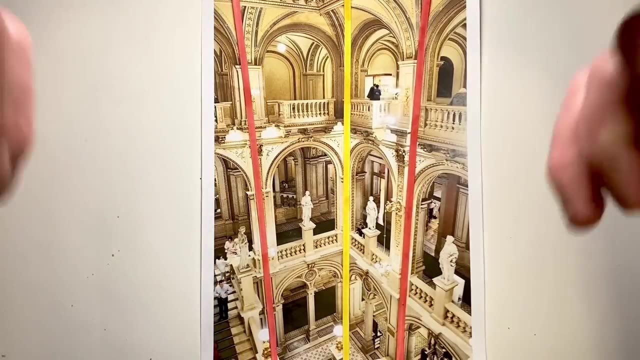 vertical again. Vertical perspective happens inside a building as well as outside, And so if we're drawing this effect, we need to make sure we angle our lines increasingly. but we also get this effect when we're looking down in an internal space as well, Exactly the same as with an. 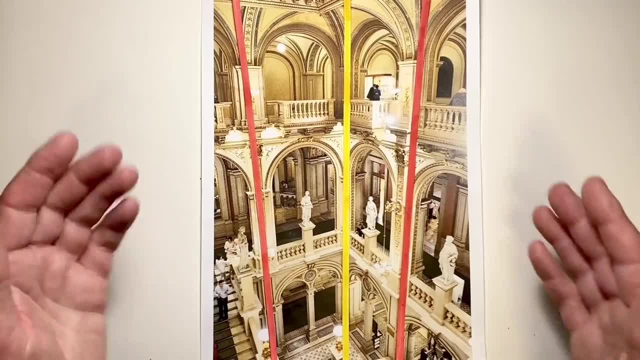 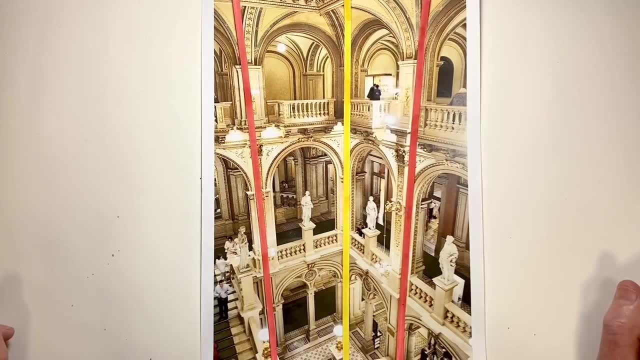 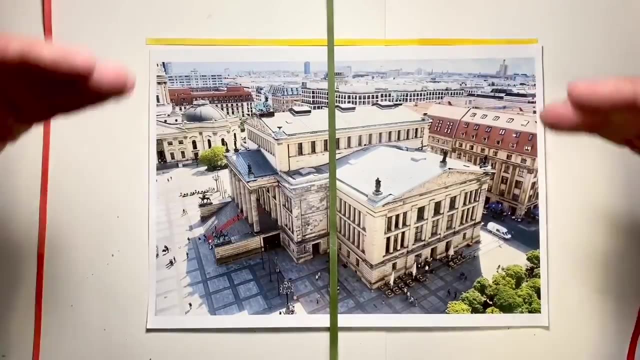 of view in three-point perspective, and so we have our one point of perspective down here, we have one point going off to the left and we have another point coming off to our right. sometimes we're very high looking down, and so horizontal eye level is actually above everything in our view, but it's the same principle. 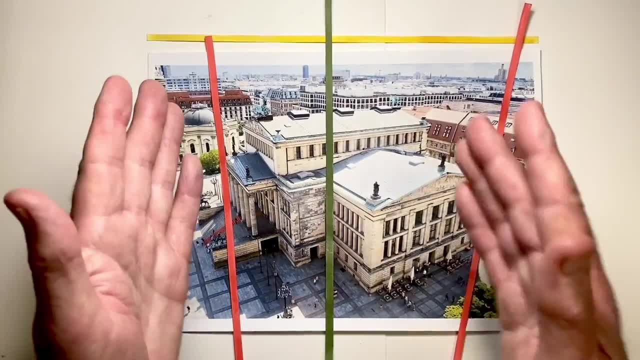 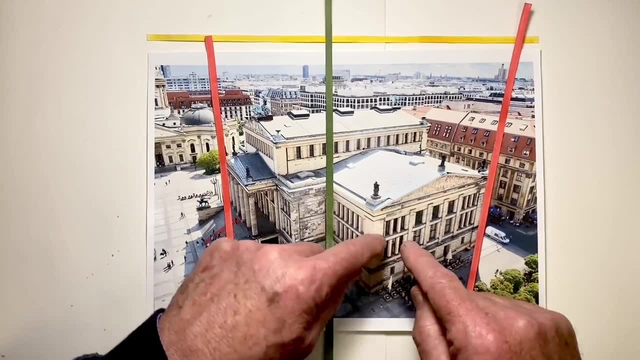 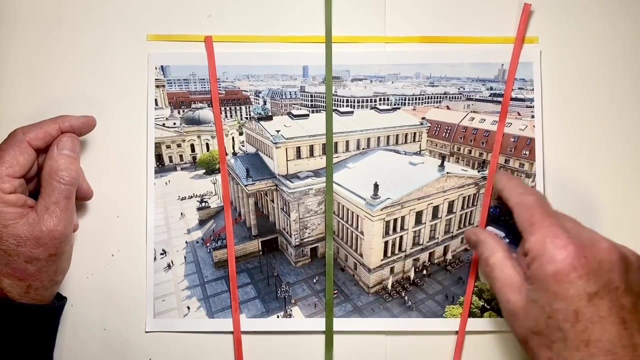 we find the vertical eye level and on that line our third point perspective will meet. and of course we can see that our first and second point perspective lines will meet on horizontal eye level, in this case quite some distance to the right. invariably, if we use a camera to take a photo, the camera exaggerates the 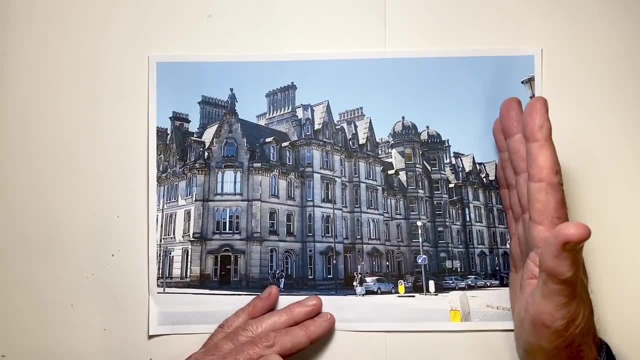 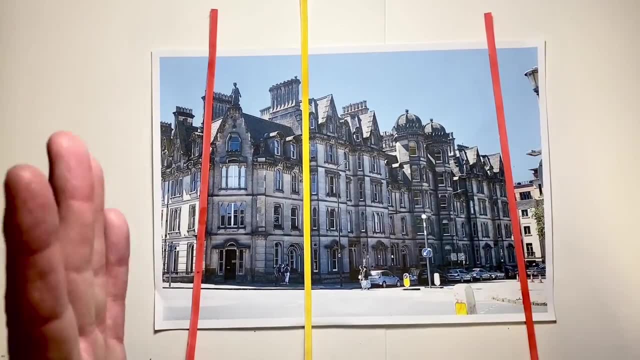 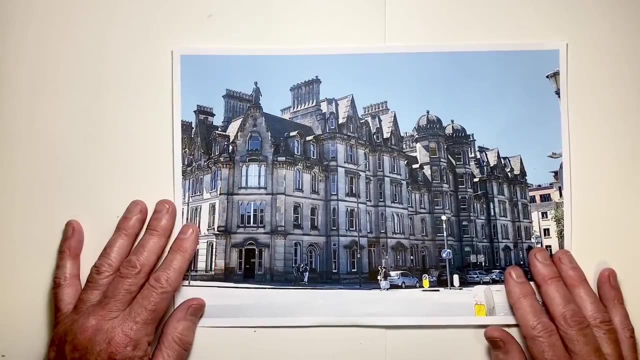 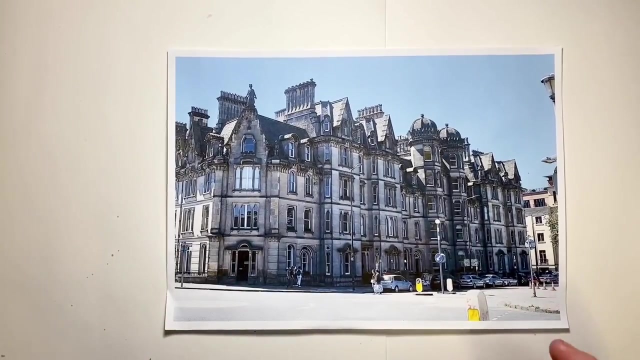 vertical perspective angles, and so we see this leaning in towards the center in situations where in real life, we wouldn't see it. and if I want to draw this scene, get the choice of actually drawing this lens distortion, or I can choose to draw it, making all of these lines vertical to reflect what I actually see, if I'm 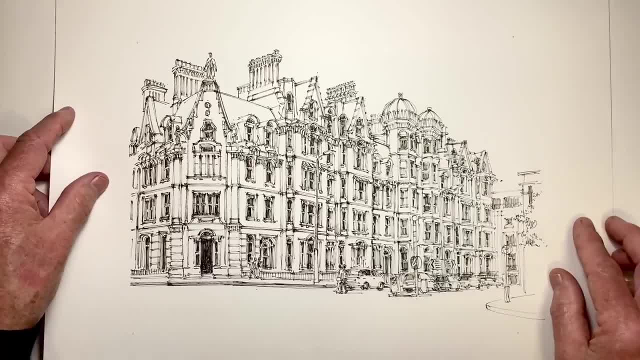 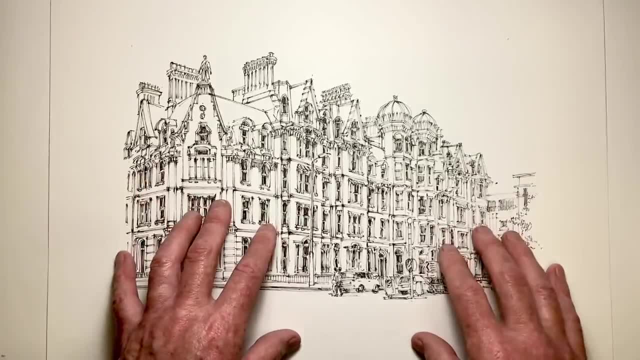 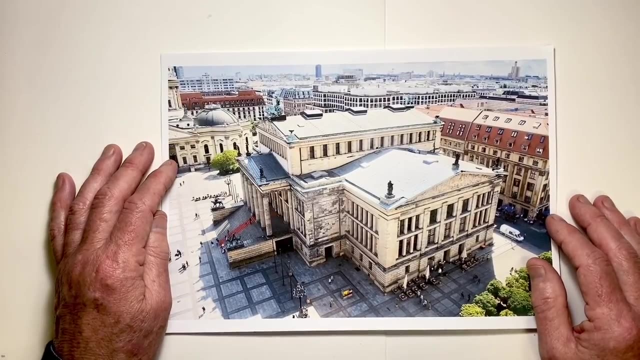 looking in the street, and that's what I chose to do with this scene. I straightened all the lines because I decided I didn't want a distortion in my drawing that I wouldn't have seen, at least in some way, in real life, and so this is three-point perspective. 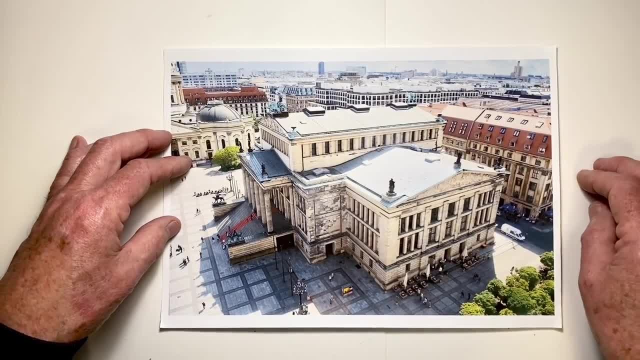 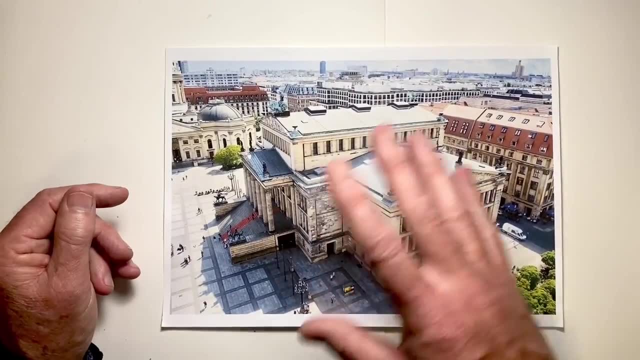 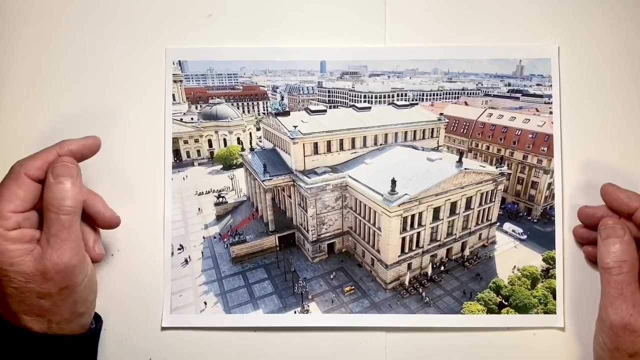 one and two points off to the left and right, and then a third point, either going downwards or upwards, depending whether we're looking down or whether we're looking up, usually happening when the object is very tall or goes down a long way and we're quite close to it. I hope this has helped you to understand the